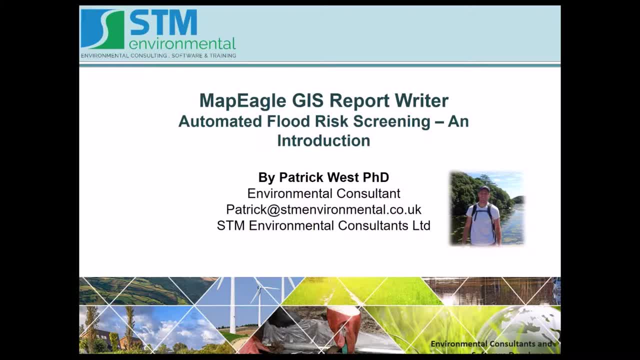 It's a slightly overcast day. I hope it's better where you are. We've got a couple people attending, just to say from current users and prospective users of the software. So the aim of this webinar is to kind of cover bases for future users and also current users in. 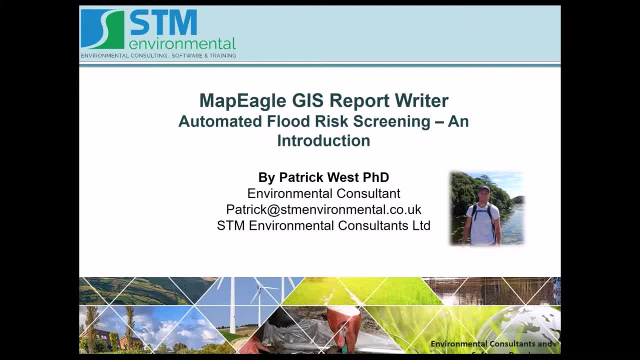 case you're not too familiar with the MapEagle system. So, as I said, my name's Patrick, I'm Patrick West, and we provide a range of environmental consulting services. So, again, this webinar is an introduction to MapEagle GIS Report Writer for automated flood risk screening. Hopefully. 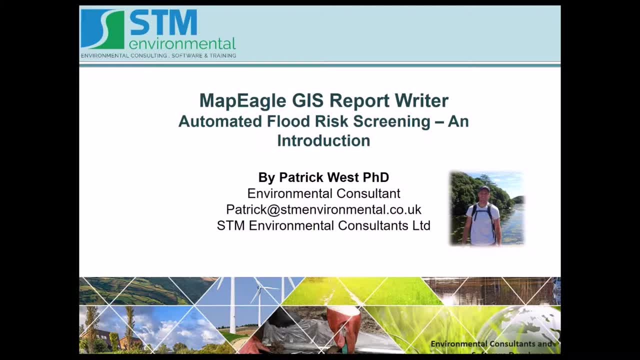 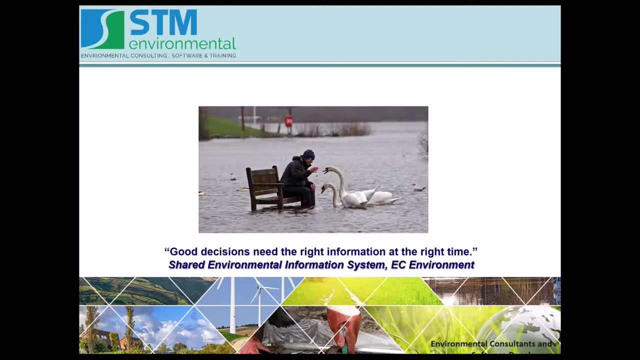 you're all working in the capacity as a flood risk officer or flood risk in the flood risk team for a local authority and hopefully we can show you how the automated report writing and screening tool can really make your workflows a bit easier And potentially more effective. So let's just get the next slide here. So sort of key to 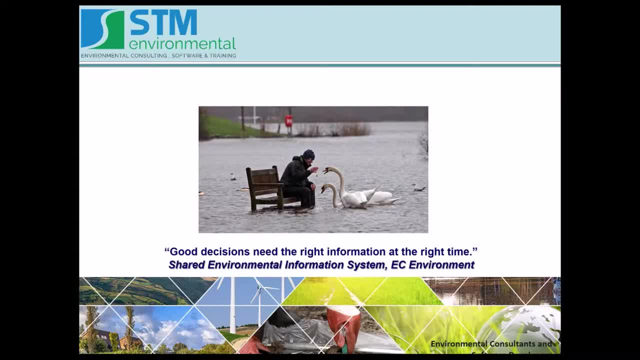 all of the reporting and screening is that you know good information and good decisions in your workflows require the right information at the right times And hopefully, as I said, we can show that the system is going to and the screening tool will make your jobs better. 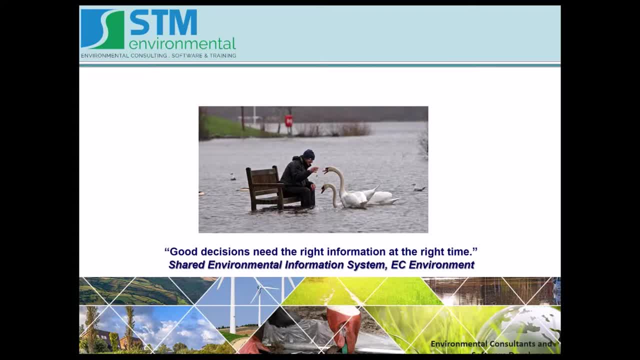 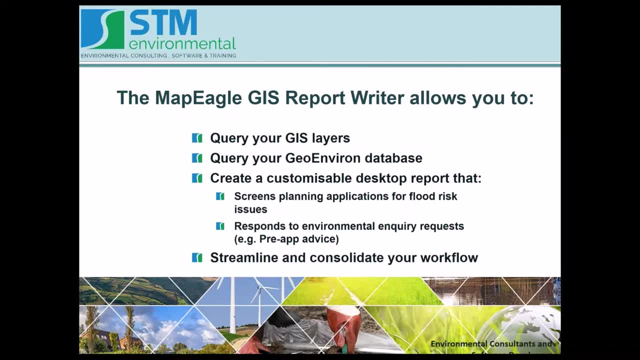 but also reduce errors that you might make when trying to search for environmental information on potential sites. So what is the report writing tool? Well, the MapEagle GIS Report Writer does a number of functions, but primarily, it allows you to query the GIS layers that you 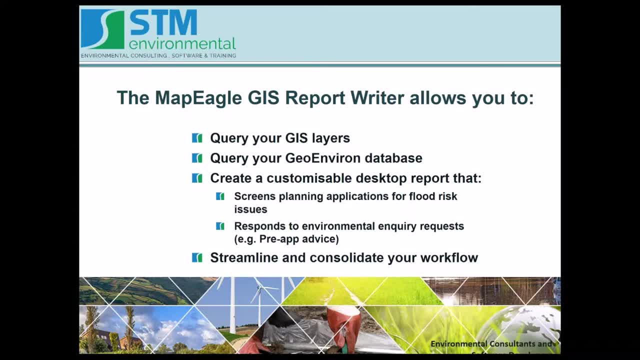 have in your GIS system, both in terms of what is there, so what flood zones, perhaps- but also any attributes associated with them, if you have them stored on your system. And that's case in point when, if you are using our GeoEnviron database system, which we 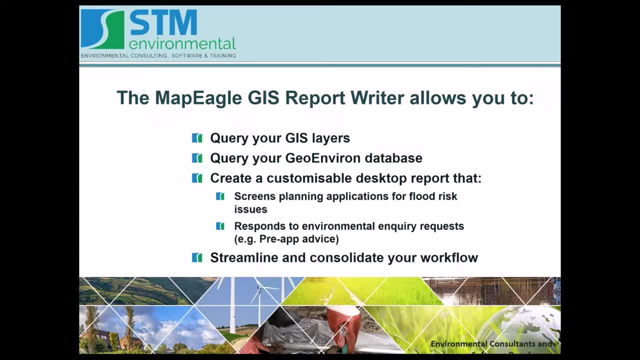 there are other webinars on that- one, which is a database system where you can manage all your environmental assets and cases. So we have an integration from our database into our GIS report writing system where you can query that information as well. So query your database for any relevant information that you so wish, And the system and the 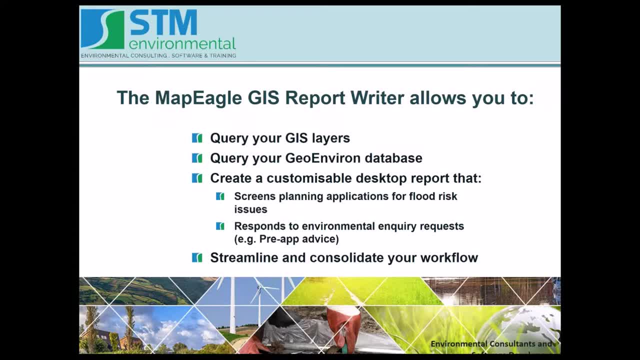 system allows you also to create a customizable desktop report. So this report allows you to maybe screen for planning applications for flood risk and potentially respond to environmental queries such as a pre-app advice. So you can use it for internal work and external work, for potentially. 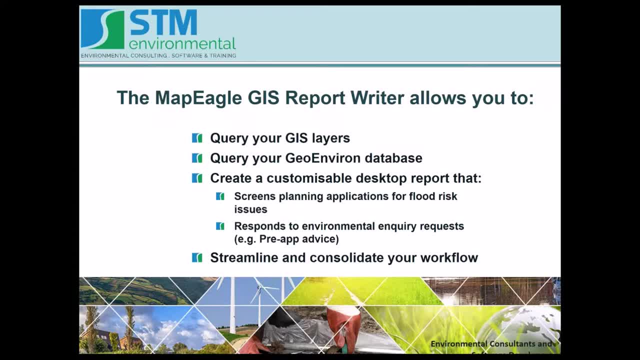 pre-app stuff And obviously the whole point is to streamline and consolidate your workflows, reduce errors by doing things in an automated fashion and obviously make things more efficient, So you don't have to spend your time clicking through all these different layers in your GIS to find out information. 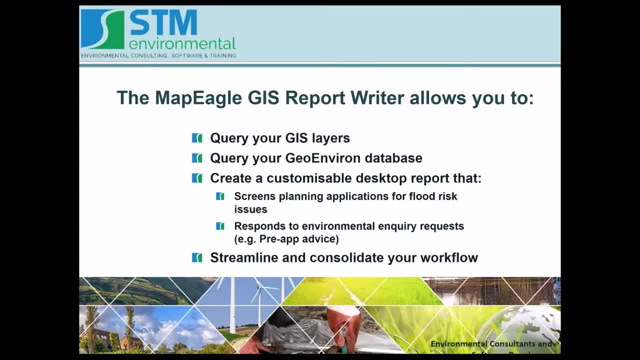 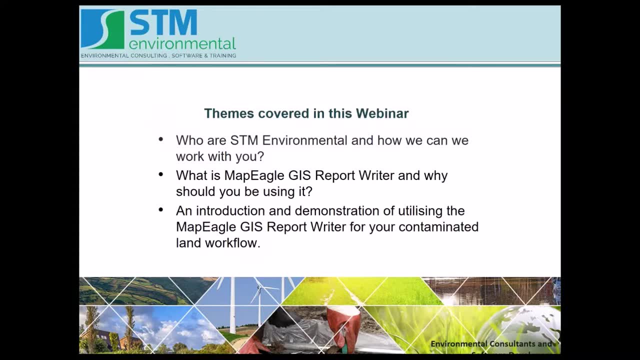 when the system and the search will do that for you. So what we're going to do in this webinar: you know who are we, STM, What is the report writer. So we'll actually go into it and maybe try and show you quickly how you would set that up and what the results look like for an automated report. 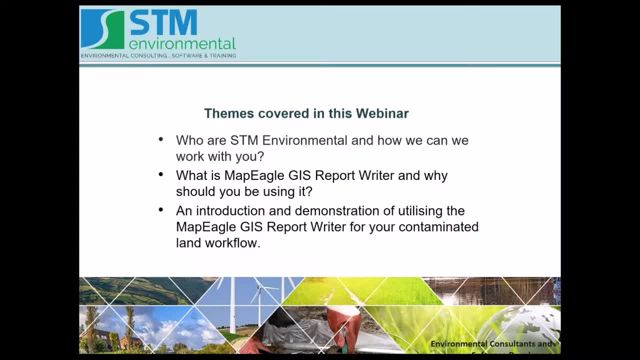 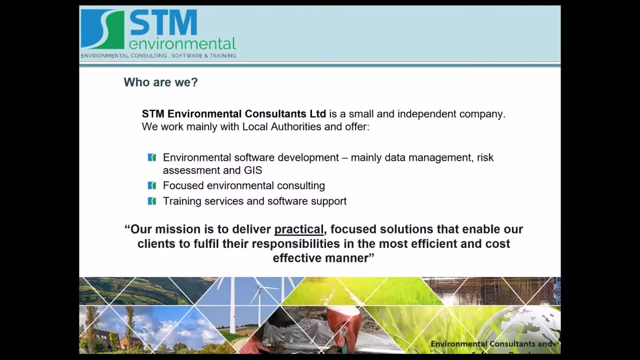 And so we've got in contaminated land here. We also provide it with a camera and a little bit of information on what we do in contaminated land, But what we mean is an instruction to how you can use it for your flood risk workflows. So 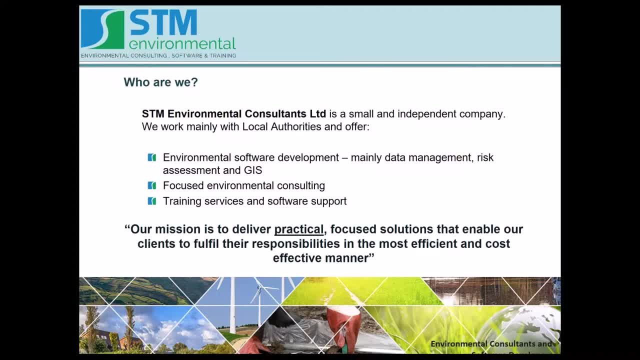 as I said, we're STM Environmental. we're a small independent consultants and we work mainly with local authorities. We provide environmental software developments and support for data management, risk management and a lot of GIS work. We also provide private environmental consulting. So we do use our system for our own private work with you know, for mainly for. 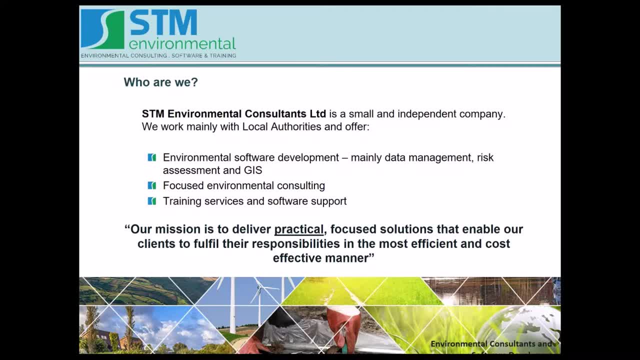 environmental purposes. So we're using it and hopefully you'll use it in a similar fashion to how we do these things as well. We also provide lots of training and services, software support, so we can help you, hopefully, with all of your environmental needs. 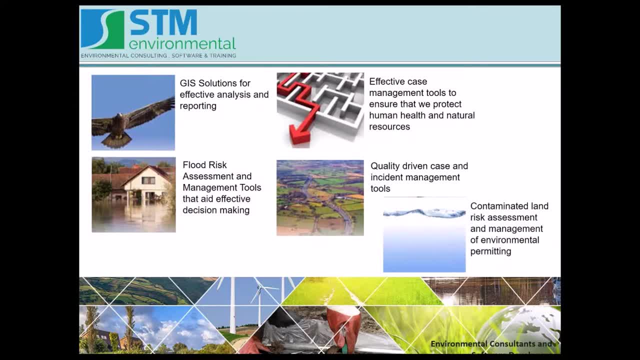 As I said, we have the GIS report writer, we have case management systems, we have database management systems. hopefully, flood risk and contaminated land risk management tools- all part of our what's called geoenviron package. I know we've got a couple of. 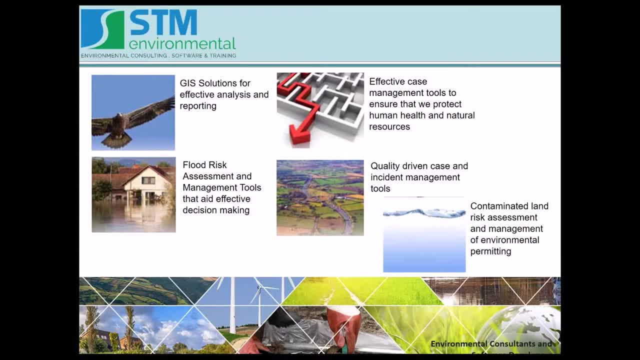 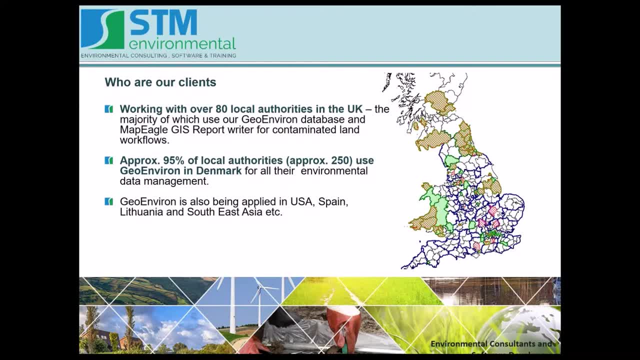 And we work across the UK with with a number of authorities, as well as most of Denmark and other and other authorities around the world, So we've got quite a lot of experience working with local authorities and and suiting their requirements in terms of their environmental management. 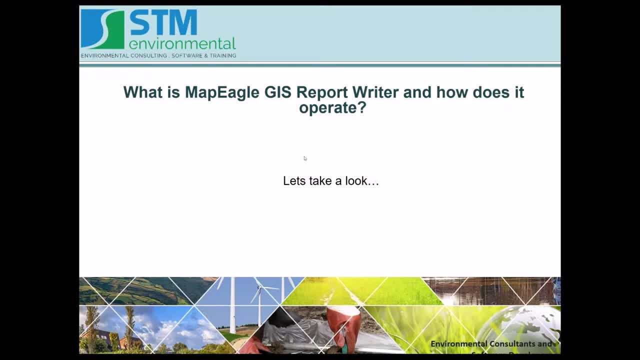 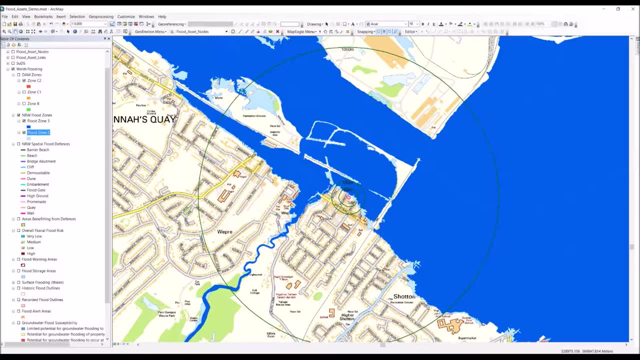 So I think we'll go to the, to the GIS reporter now, And if I just exit the webinar, the PowerPoint, and we'll go. Okay, so I've got ArcGIS open here. We just to say: we, you know, we cater the, the software. 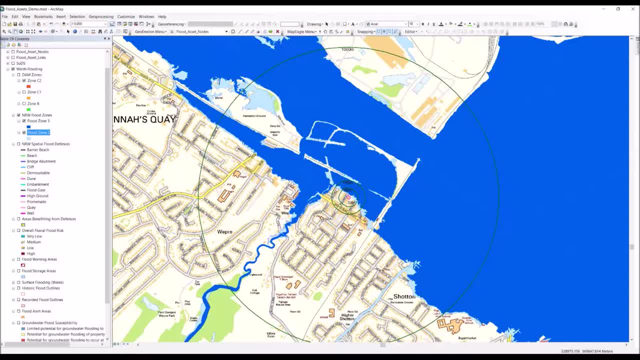 caters for most GIS systems now, whether you're using map info, QGIS or GGP, I think, I think we can do on that one, And we also provide our own through map x as well. So So don't worry, whatever your GIS is we, it's suitable for any any sort of GIS system, So that hopefully this is a 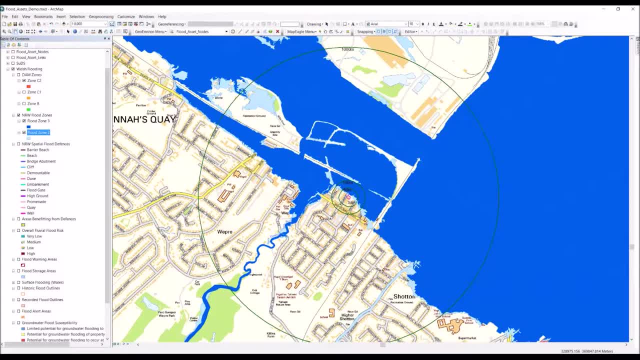 sort of similar sort of GIS setup that you might have in your, in your authority, with with a site somewhere in a particular flood zone, or you want to work out whether it's near a flood zone and what other potential in geo environmental layers that you want to look for. So I've made up. 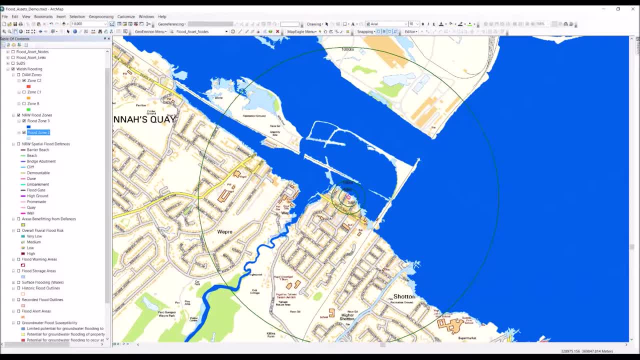 an example here. it's a site in Flintshire in North Wales And we can see that this site is. this isn't a particular, I've just drawn a random polygon here- But there's a site that's near the river Dee and it's potentially in the flood zone. 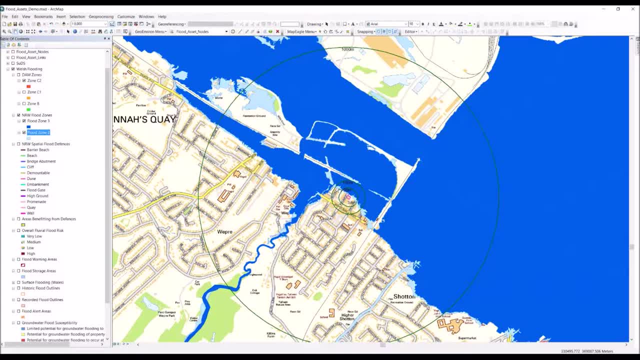 we want to know what information is near that site- and historic records perhaps what? what does it benefit from? defenses? what are the defenses? but potentially, as you can see on on the left hand side, I've got all of our layers freely available from Natural Resource Wales, but potentially you have your own layers. 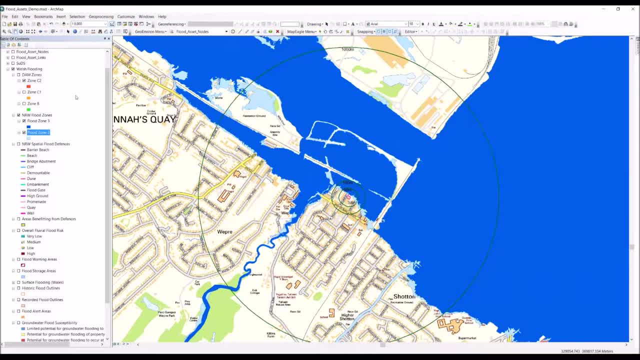 specific to your local authority, whether that's assets that you have for your internal work or it might be recorded flood events that you have that might not be available through government websites. so, as I said, any any sort of critical layers that you want to search for, you can have them loaded in. but 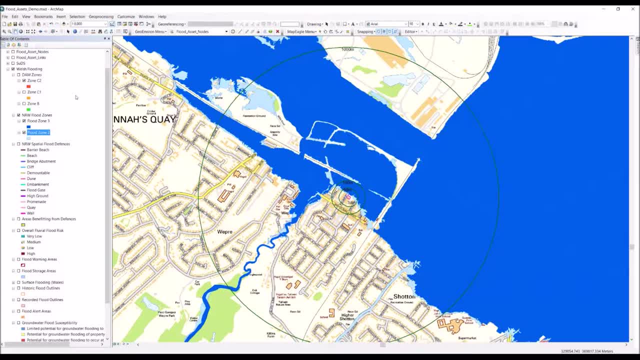 obviously, to search all these layers manually might take some time. it also might have some associated error, you might miss things, and the idea behind the tool is to search through those, those layers for you and give you a report, depending on the complexity of of what, what the outcome is. so to hopefully. 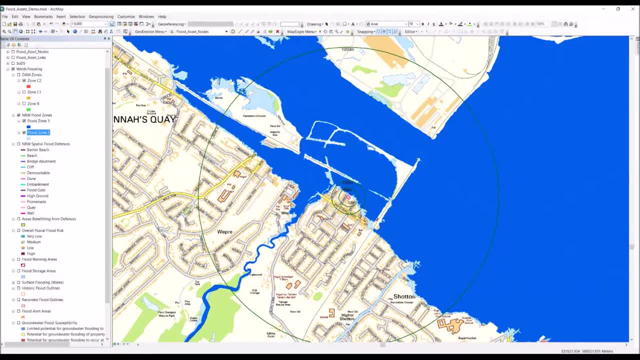 streamline your advice. so, as again what I said, if you look on our GIS we have at the top here- I'll just right click there- we have a map eagle menu where the mouse is just hanging there. that's. that's where we basically start from, start our search from, and we can either search, search the layers and and just. 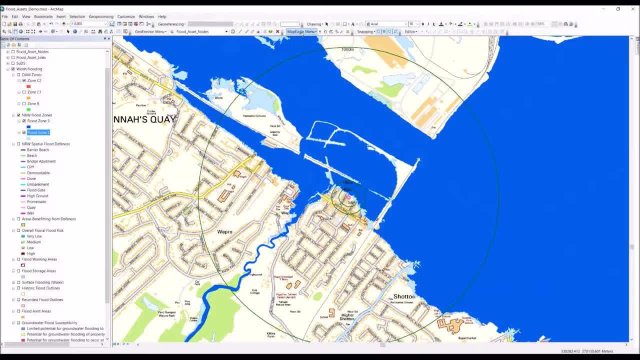 have a look at what's of what's around that site within a prescribed buffer distance, or we can go go ahead and actually make a make a full report. so I'll show you an example of this site here. so, for example, say someone has submitted a planning application and you've been asked to flag any any 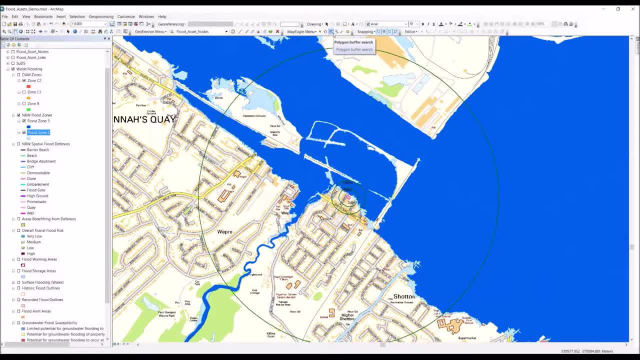 potential concerns in terms of the flood risk side of things and you'd obviously have the layers that you want in your contents page of your GIS. so the report writer what? the search tool starts by obviously searching those layers and that is totally customizable so you can choose what layers you want it to search. 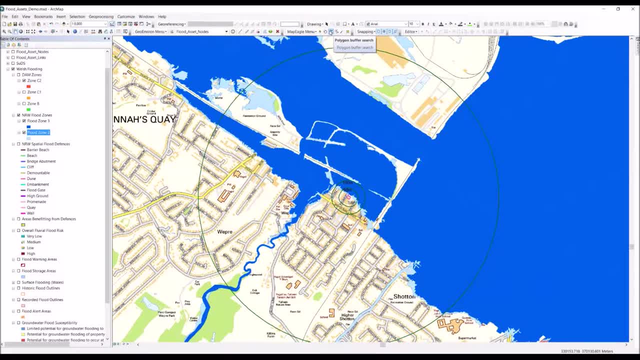 for different projects. so you might have a potentially a pre-application advice layer project where you want it to search a number of layers, or maybe just a couple of them to to to give that that applicant some advice. or you might have an internal one where you want to go into. 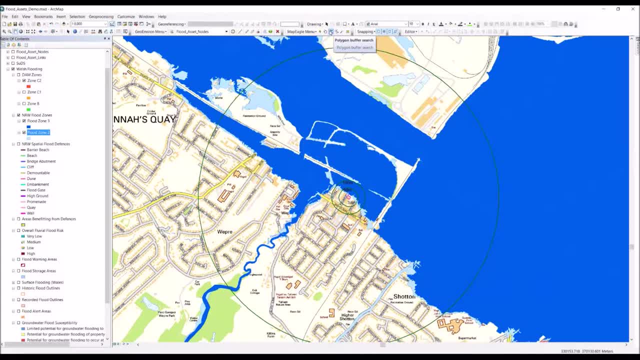 more detail and search through a whole range of layers to give you a broader picture. so you can customize that, which I'll show you how to do shortly. so we begin by. you can do a polygon buffer search where you can. you can choose this: the shape of the of the feature that you want to search around. so normally you 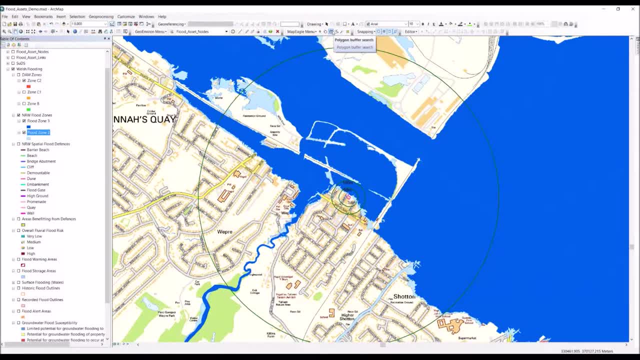 would draw, say, a polygon round a site, or you might have a pre-loaded site which is a particular shape file via your GIS, so I via your case management database, if you're using that system. so we click the polygon buffer search gives me the option here to repeat the. 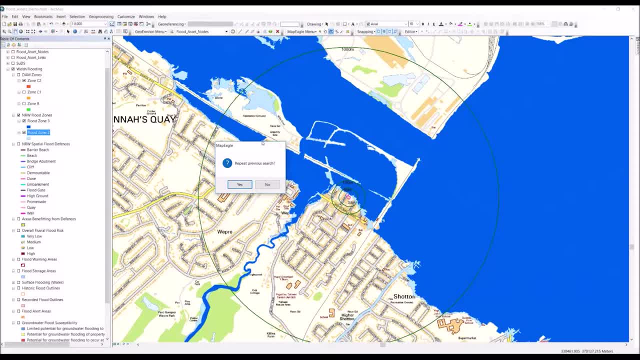 previous search, which is the one shown in the image. so we'll say, yeah, we'll repeat that search. I want to know what the what are the potential flood risks associated with that, with that new site there. someone might want to build a bungalow or redevelop that site. so yes, it's repeat that search and we'll search. 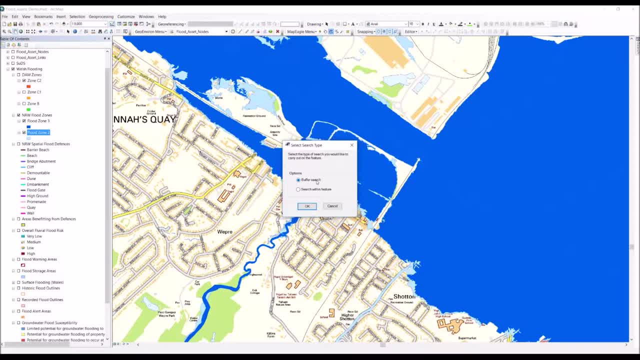 within the buffer buffer features so we can search within a feature. if you've got a very large site, you might just want to look at what's in there, or you can search within a, as I said, prescribed buffer distance and that that search distance will can be customized depending on your layers. so 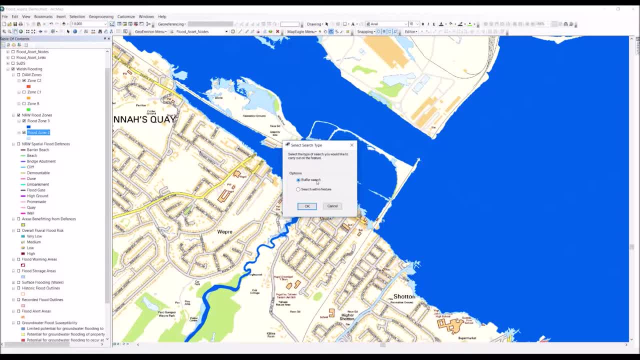 for the example I'll show here is that it search, is quite in quite a close proximity, for four things like local, any local flood risk or flood records and flood zones. but it might search for a ride at wider radius for your flood defenses and which, obviously, and any local rivers as well, which might be up to 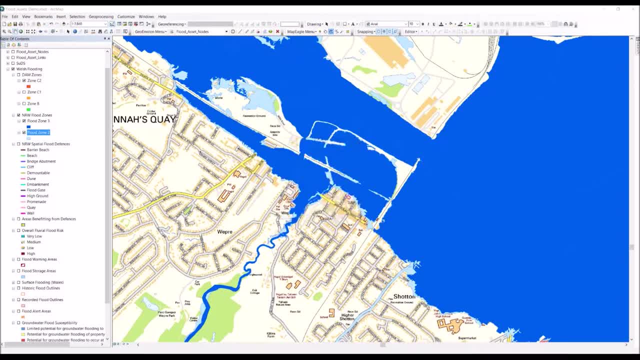 maybe a kilometer away. So we we okay on that search And what the system then does takes a quick second to get going as it will search through all the layers on our contents pane, on our on the left of the project here, And it will search through the ones that 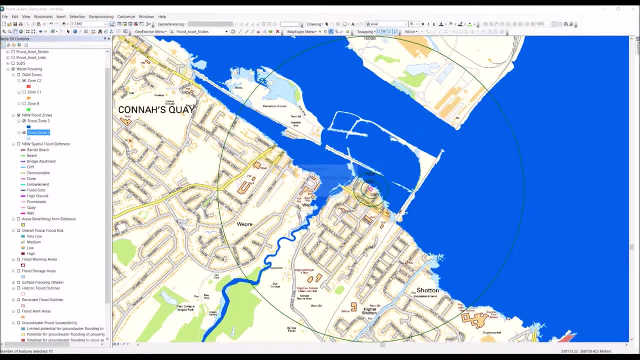 I've told it to search through. as you can see, it's popping up now, So it's it's quite quick on this one. I've got the, I've got the, the data stored locally, So it's really really rapid in that. 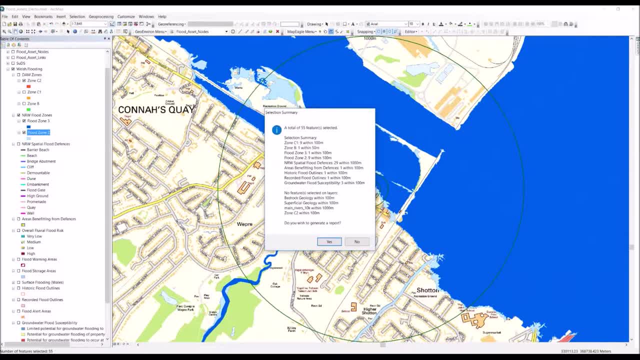 respect And it's gone through the layers that I've asked for. So you know flood zones, any spatial defences, areas benefiting from flood defences, any records of flooding, and I've got some groundwater susceptibility here Also. 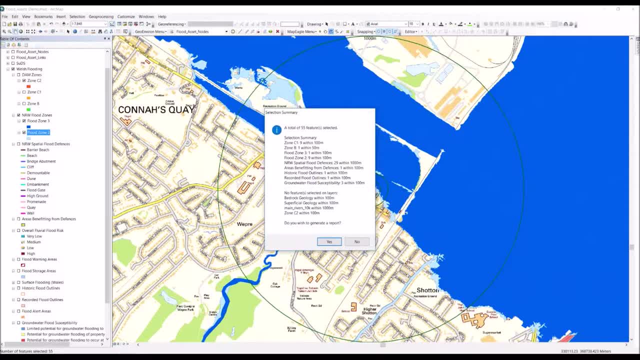 obviously if you're. if you're not aware, in Wales they have a development advice map which characterises flood zones into defended and undefended Zones three and and two. So we've got zones zone C one and be there if you're. if you're not familiar with that designation in 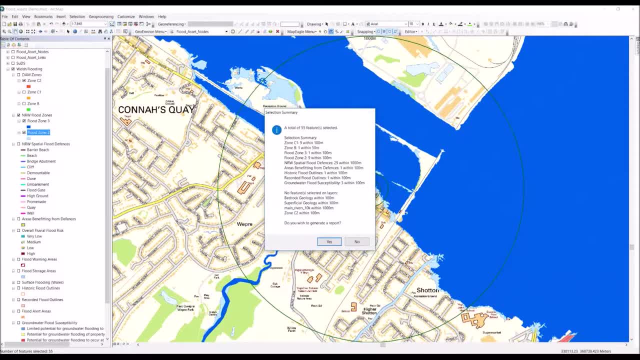 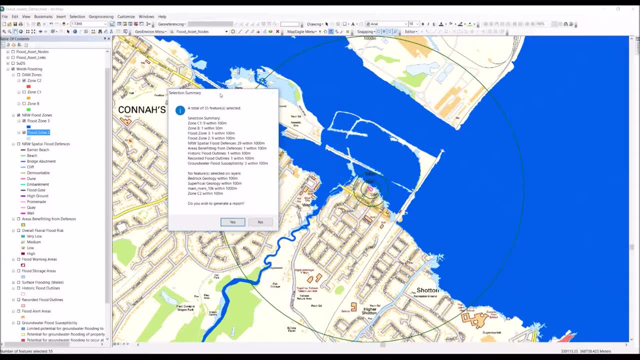 Wales. So you know that was pretty quick- certainly quicker than I could have searched it for myself- to find out that information, And so you might be happy with that- And to find that there's a. you know, you've got your sites and you've found. 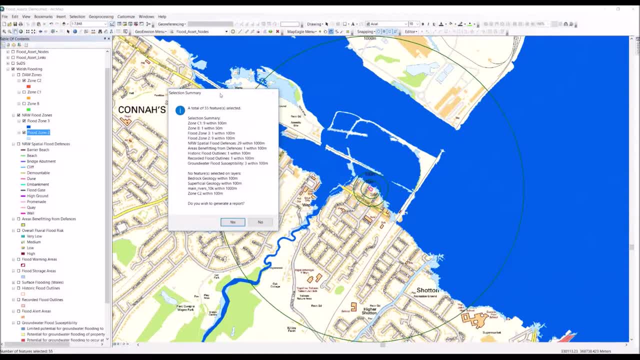 a number of different features and it tells you obviously the distance, And so that might flag up your concerns And you can- you can quite quickly report back and say no, that site is within 50 metres of this zone, or it's, it's not within that distance. 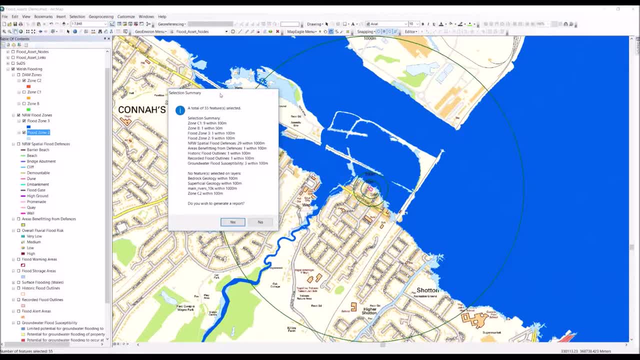 So as a as a very quick checking tool that's, that's quite effective for doing that. And I'll just reiterate: you know you can choose the layers that you wanted to search. So in this instance there isn't actually records of any bedrock or 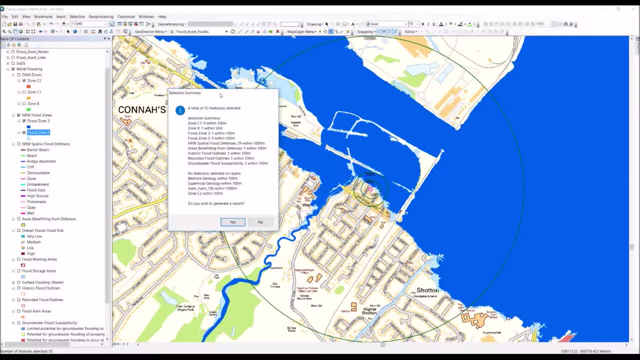 superficial geology, But you might have other other geo, environmental layers that you think are critical to your, to your kind of initial assessment. So we could, as I said, we could stop there and just report back, or we would. we might want to actually generate a. 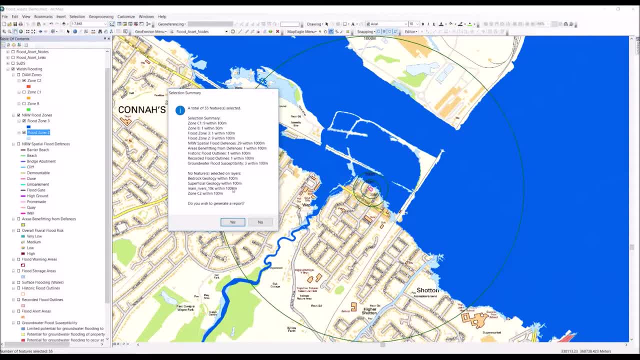 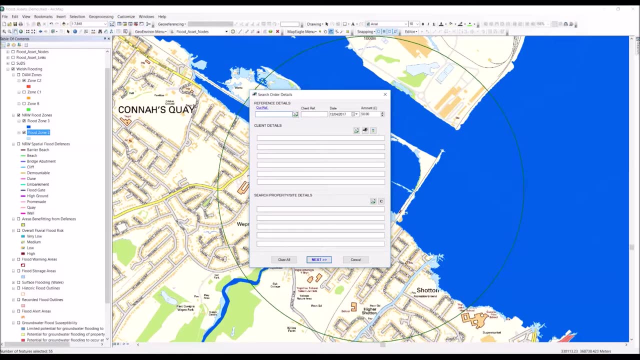 report on that information to potentially submit to a colleague or to an applicant in terms of pre app. So I'll click generate reports. Yes, and this is quite a fun feature. So if you are potentially, you know, providing this as a pre application, 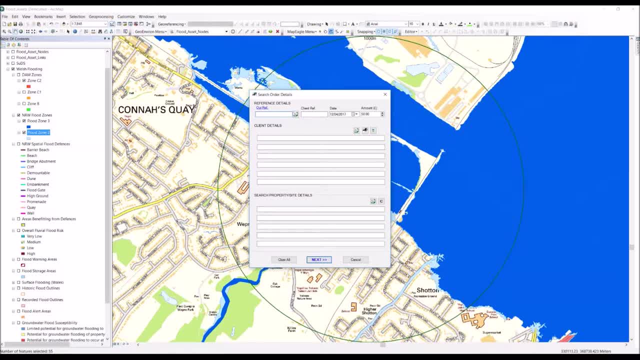 advice, or you might have a particular internal format for how you, how you do your reporting. or you maybe don't have it, but you think that it might be suitable way to way to progress. you can, we have a system where you can obviously put your clients. 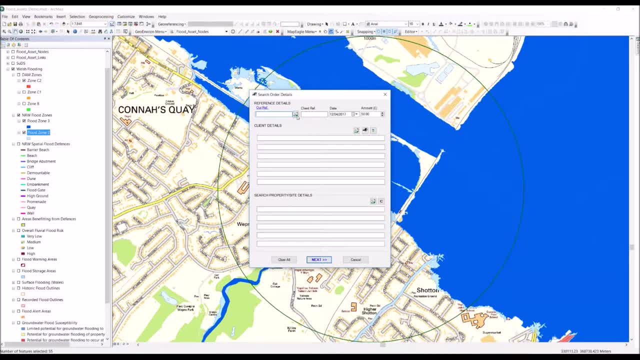 details and the property details on this option here And you see the icon there: G, the little G icon. that's the link back to our database system that we also provide And so you can actually import references from that if it's a for a particular site from. 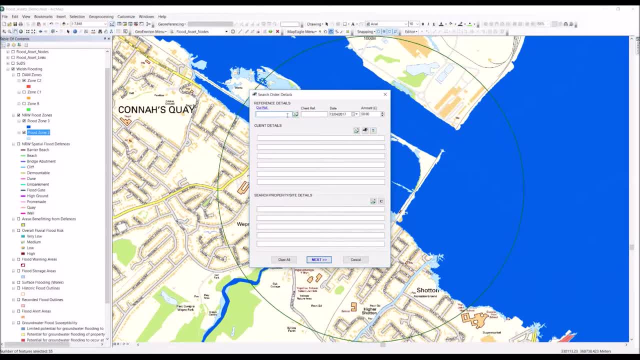 your database. So I'll make an example here And call it flood screen report 001.. And we'll call the client details myself. And these details they populate within the report and through bookmarks. so you can, so you know you can. 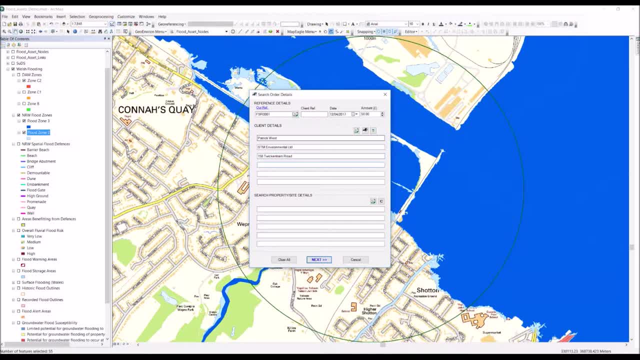 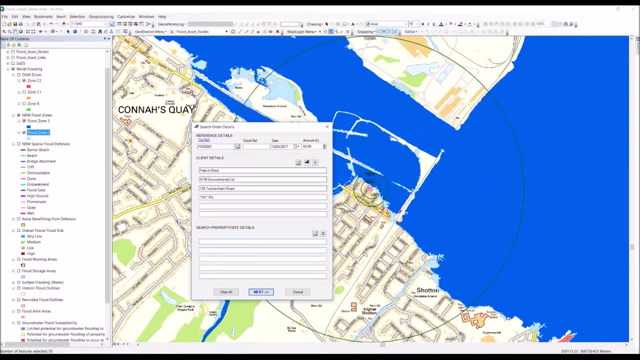 basically have the whole report that comes out automated. So I've just put our address here. we're based in West London, as I said. I don't know if you might. you might know this area And I'll make up a property address. it's somewhere in Connors Quay in in. 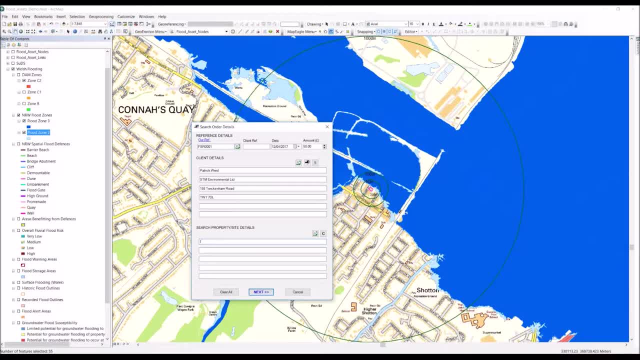 in northern Wales, So we'll call it. I don't know one D side road, I don't know if that's a street, but it's doesn't really matter at this moment, And it's in Connors Quay And that's. 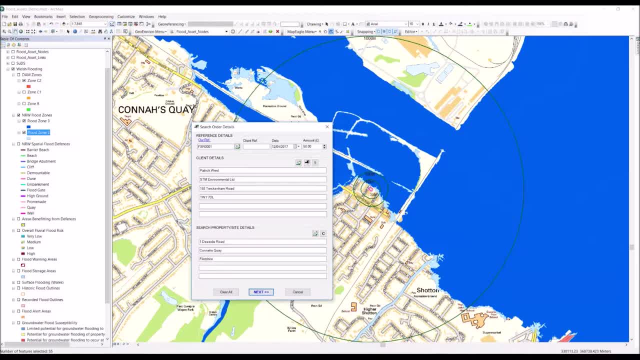 Flintshire. So bear with me here. make up a postcode, WW one one, a little bit, Okay so. and as I said you can, you can import these details from your database if you're using that To make that even quicker. There's obviously a cost at the top there If you are. 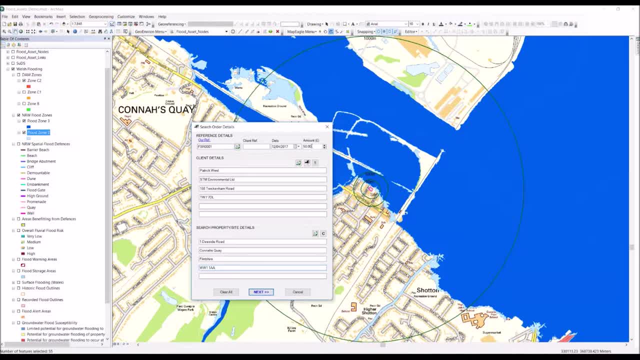 providing it for any pre app or hope to maybe provide pre app detailed advice or information for for private clients you can obviously put your cost in there, the date and a client reference, So hopefully covers all of your kind of internal nomenclature for. 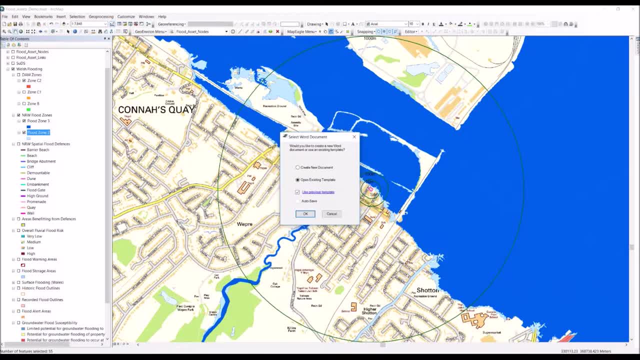 you how you report these, these things. So we click Next And then it. then it's going to basically go in and generate a report. So I think what I'll do is I'll show you the the output report that it looks like first. So if I just get a, 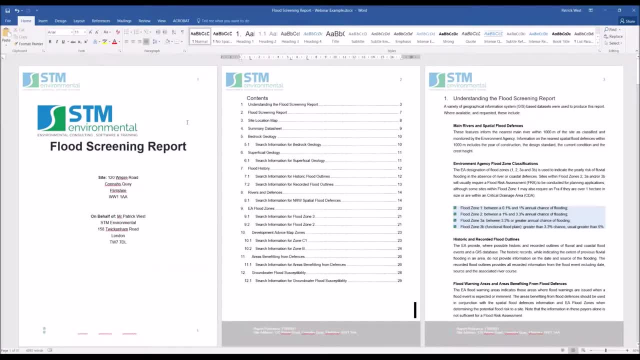 screening report up and hopefully you can see that. Okay, there we go. So this is. this is what I did earlier. In true Blue Peter fashion, I've made a flood screen reports for this same site And everything you can see there is has been automated, And so I. this probably took 10 minutes. 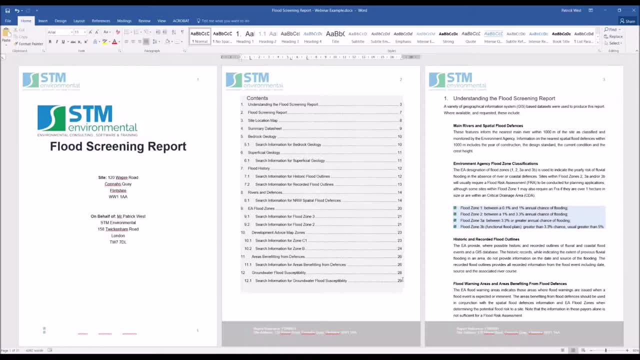 for the system to run in total, from finding the site to running report, And obviously you can customize this and I'll show you the template for that in a second. So on the first page on the left, it's got the details that we just entered of the 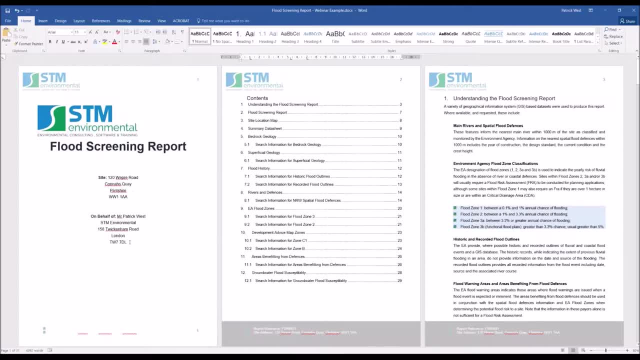 client and the site. There's obviously could be your internal details if you want table of contents and some preamble about this screening report, So this might be your, your flood screen report, and you can customize what information you want to say there about flood zones and any. 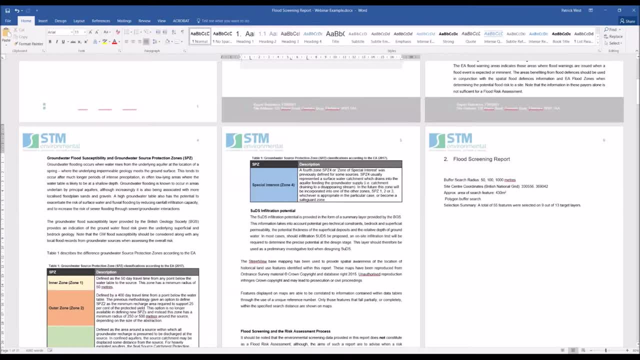 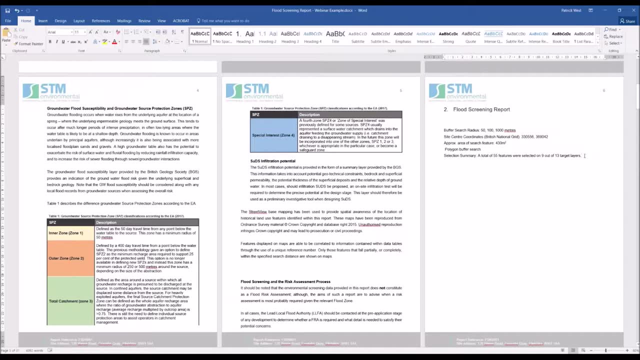 any limitations in data, etc. So then, if we we can see that it gives a bit on the on the far right there, it gives some information about what the search was And you can again customize all that information: the buffers that it searched, the grid reference of. 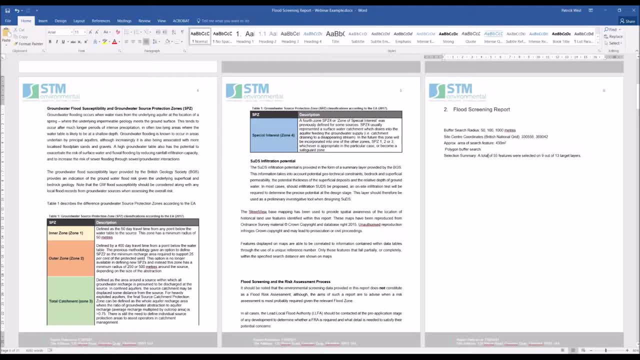 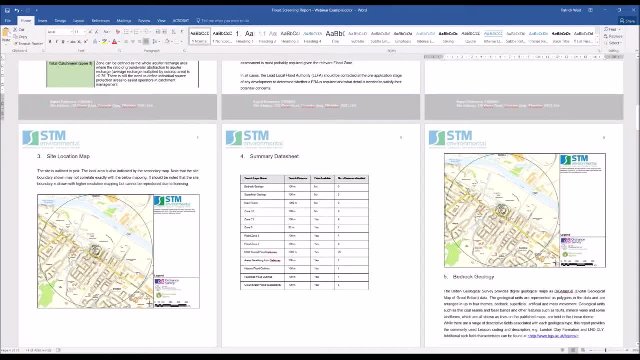 the sites which is useful, the area of the feature and how many features that you found in total, and an option, If we just let the the webinar scroll with me because I'm a slightly ahead, It gives a site location map on the file on the far left there. 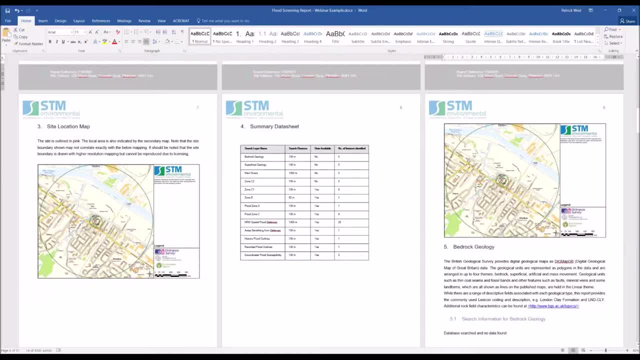 of where that site was And you can have all those, all the layers that you're searching, pop up at once if you like to show that you might have a number of flood assets, your culvert stitches, etc. For any internal work that you want to pop up and 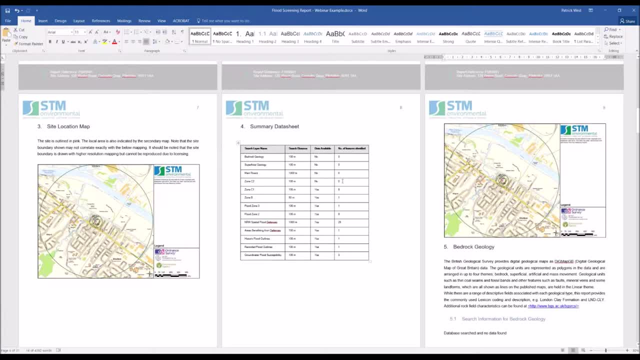 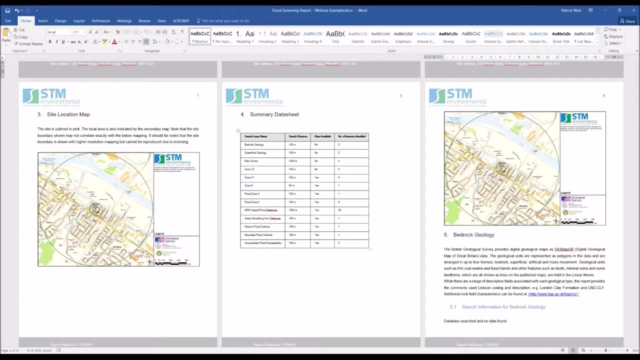 show on that, on that screen there And then middle page, here we get a summary data sheet So it summarizes, if you, if you want it to produce a summary, what, what layers it's found, And so that summary report up to that page. 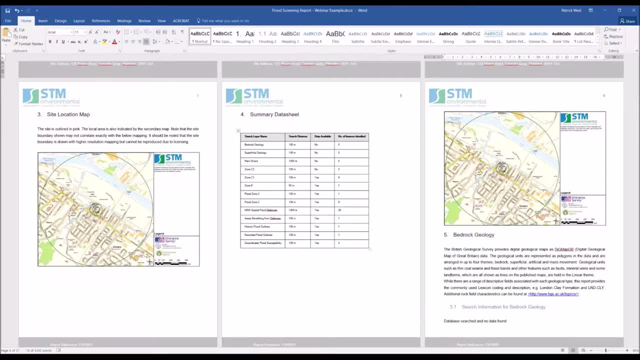 eight there. So the summary data sheet. that can. that might be all that you want. you might just want to show all of the features and just a list there in the table, which will go back to the writer writer in a second and show you that, But you can. 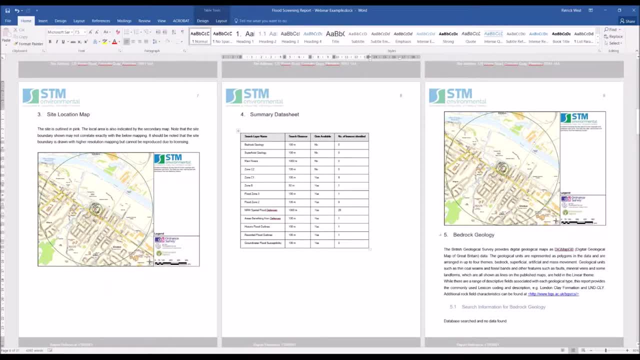 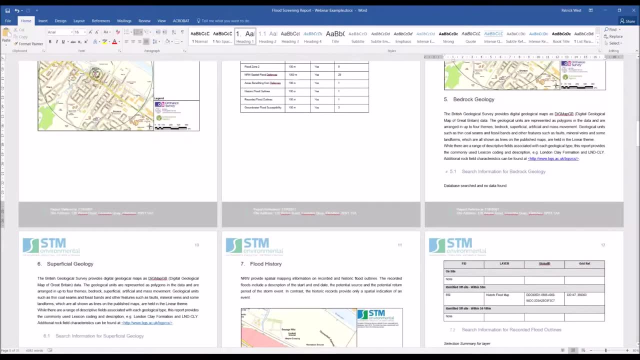 continue and you can output a detailed report depending on the layers you want to search. So we- this is an example that I've made here So that might search the bedrock geology. There's no records, unfortunately this in this part of part of Wales that I have in in our in my GIS, but 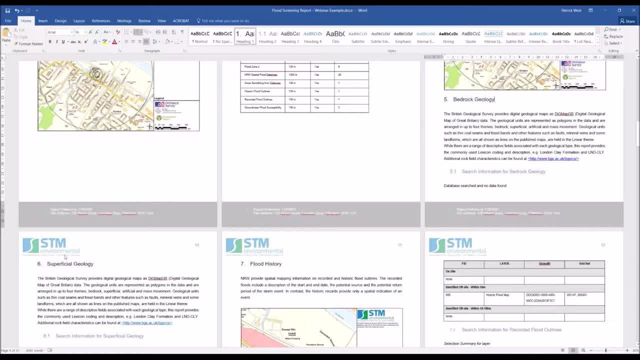 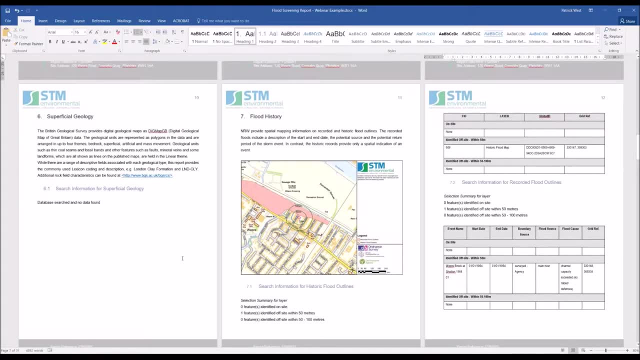 you if you were doing in England. I know that you've got most of the land covered there And some more examples here: flood history. So it's it's picked the layer there. there's a record and it's within 50 meters. that might be a concern. 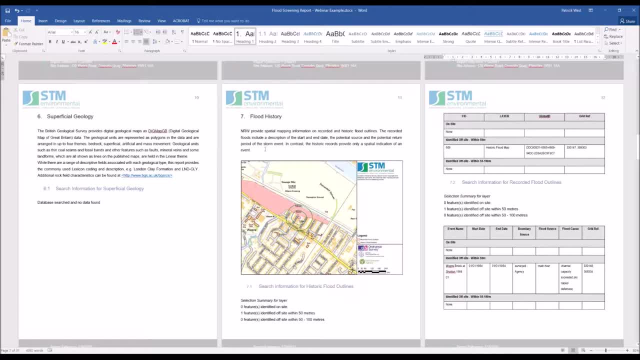 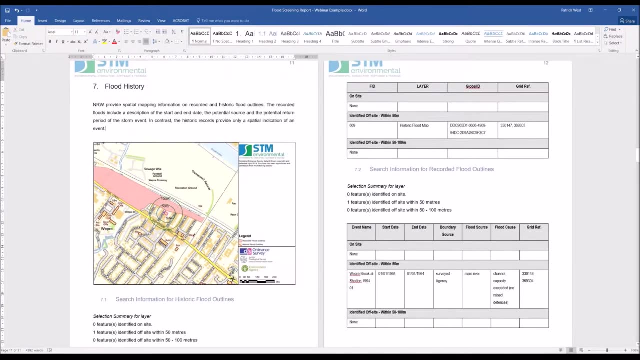 of yours that has flooded, and and then you, the system will give you a map And the search information that it's found within that, within those buffer radiuses. So if you look at the table, maybe I'll just make that a bit bigger actually, So you can see. on the, on the. 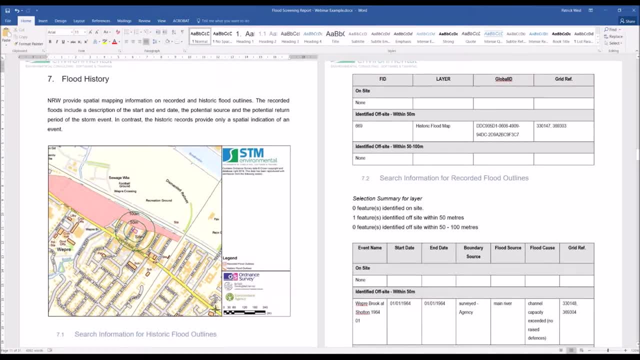 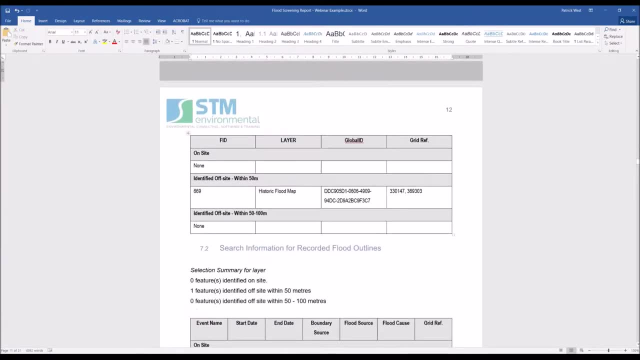 screen. I've got quite a large screen so you might not be able to see the table here, But bear with me. So that's, that's the map, And then it will give you the the layer information. So we'll output the attributes for that, for that layer, that the 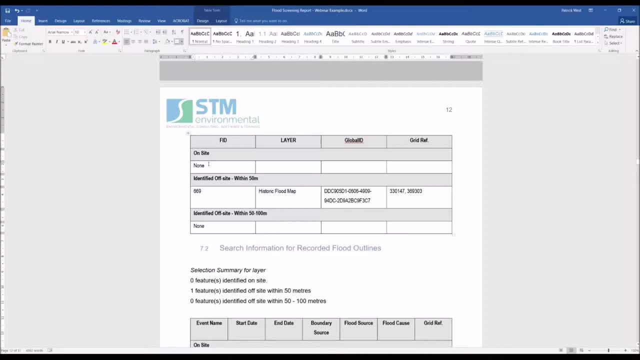 system has found. So hasn't found any flooding on site, As you can see there, but it's found a feature off site within 50 meters. Some reason it hasn't found one within from 50 to 150. But we know that from the mapping that there is that. so 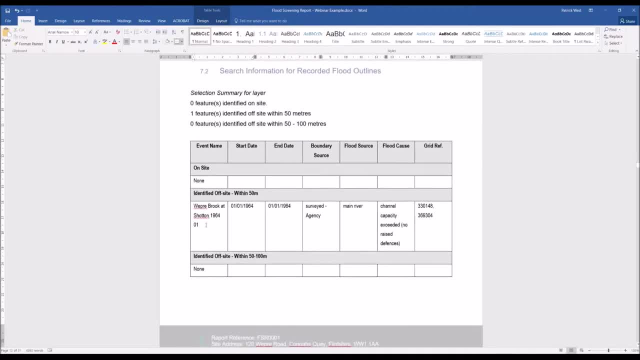 that was a historic flooding, And then we've got some recorded flooding, And so you can, you can choose what, what attributes are extracted from the from the search. So in this instance we've got for for: flood event start date, end date, saw for. 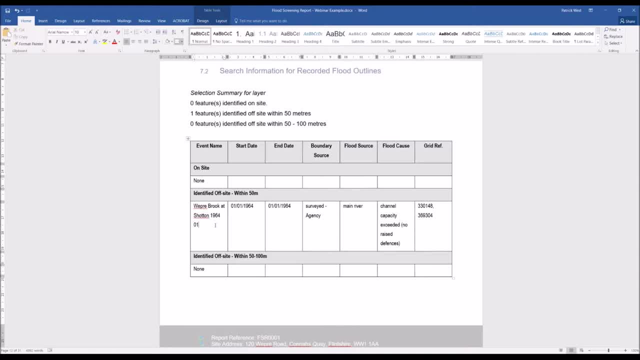 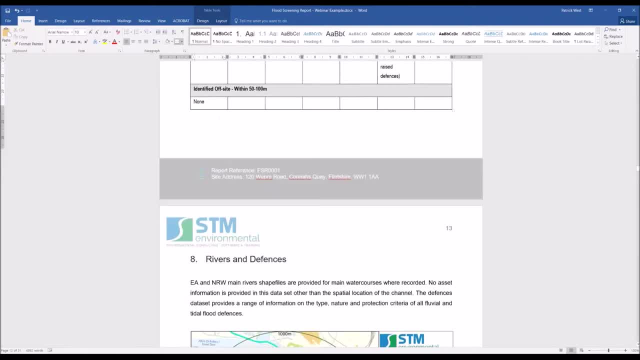 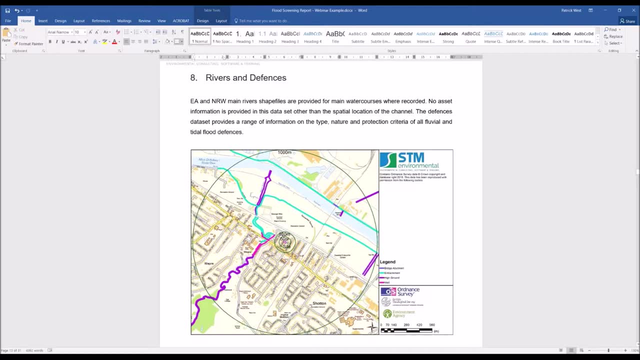 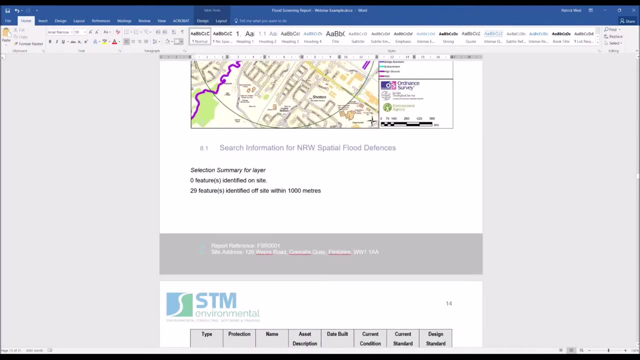 choose what appears and what doesn't appear in your, in your data table there, And I'll just quickly scroll through another example. maybe you have some defenses you want to look at And again, that's that's a freely available layer that I've, that I've got from NRW And so that's not a good looking. 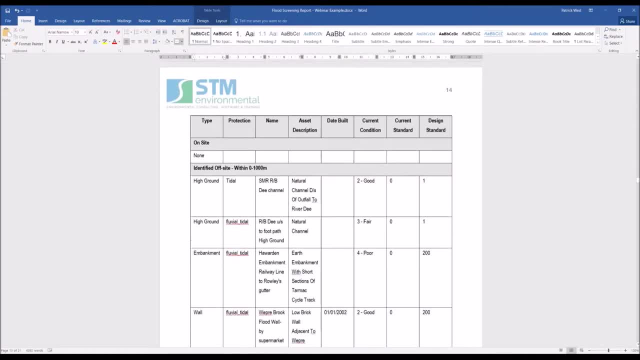 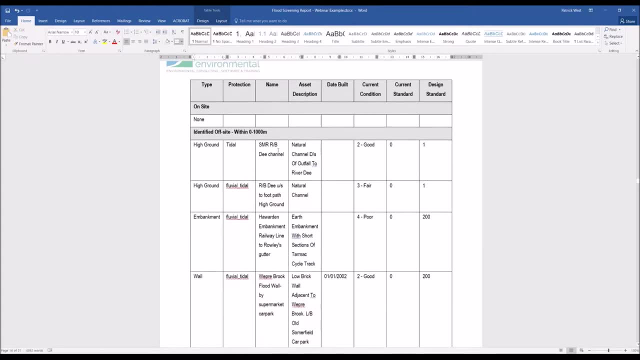 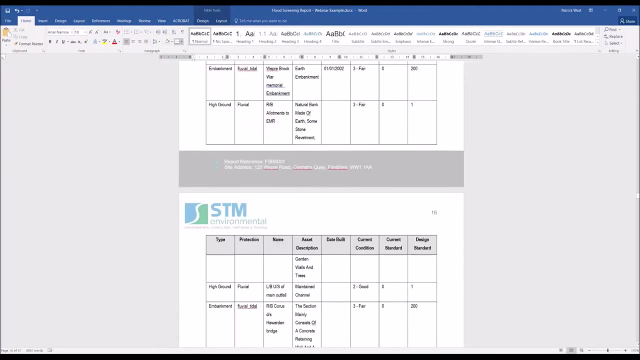 map to see where, where those defenses are And, again, an attribute table of all those defenses within your, within your. so we've searched within a thousand meters here, which is which is quite large. so we're going to have a lot of information about, um, all those, all those assets. so, um, and i won't, i won't go for. 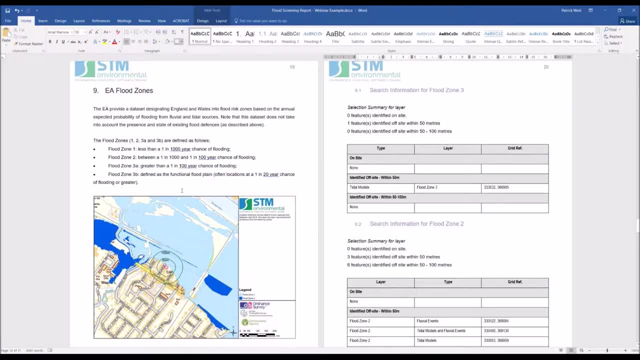 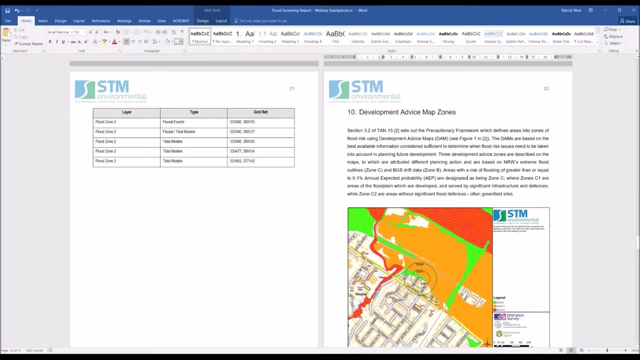 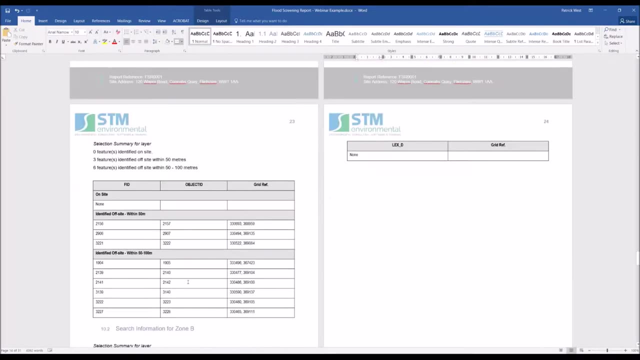 everything. but, as again you know, we've got um a flood zone layer. again, this is all customizable um. it's ea flood zones. if you're in wales, we've got your dam zones, so zone c1, c2 and b? um and their associated attribute information on the tables below. so and that's all automated. 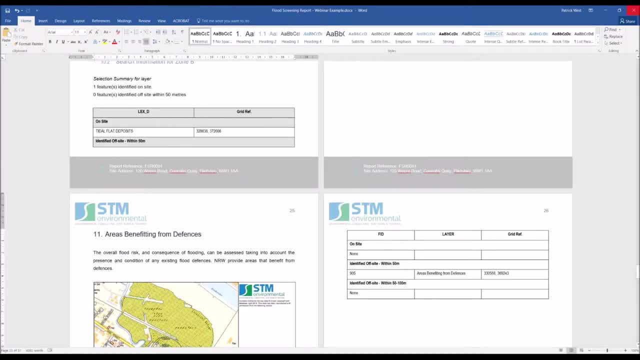 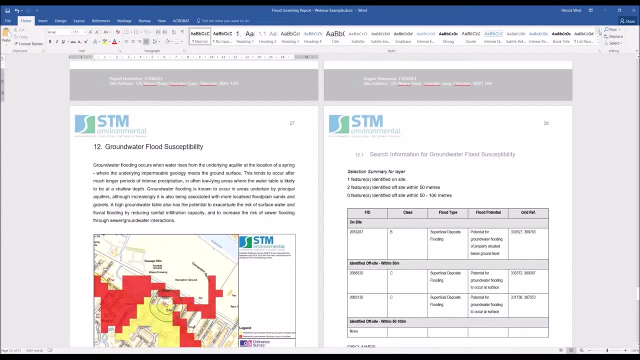 report. as i said, it takes maybe 10 minutes. um, it depends on how many layers you want to go through. so if we go back to the gis report writer now. so that's the, that's the, the output that we want to get and we will get from the report. um, i'll just quickly close that one. so we're back in our gis. 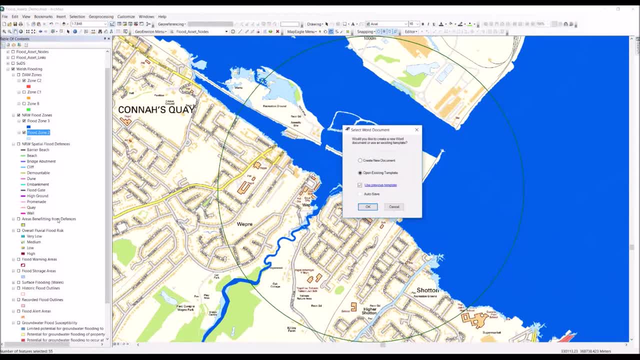 now and we did the search of the layers. we've asked to run a report and the report, open, runs in a template that you, you predefined. so that's how we- uh, how we got that one to look so nice and we've got some really good examples in some authorities of some some great looking templates. 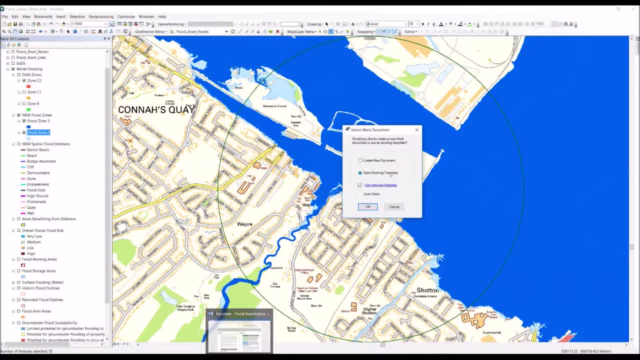 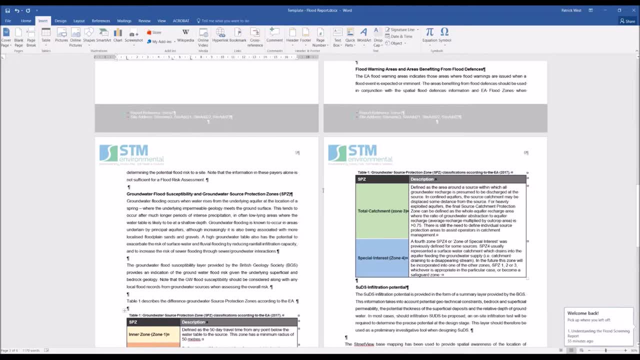 and really helpful, helpful bits. so, um, we can open an existing template or we can create a new document. um, so we can click use previous template and that shows you what your template is. so this is the template that i have, um with the with the relevant bookmarks to bookmark the client address. 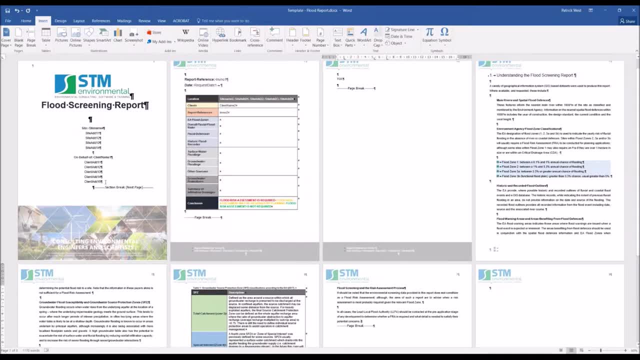 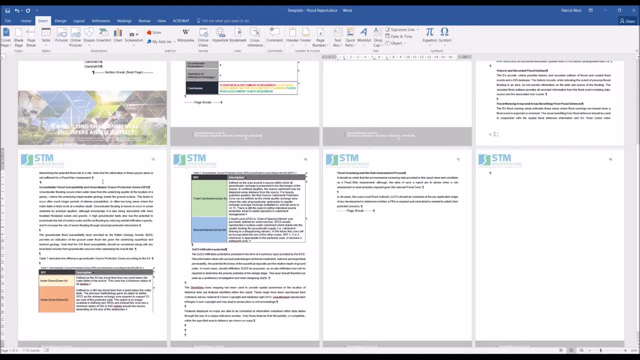 and the, the, the reference for the, for the search, etc. and the report populates that template at the end of the um, at the end of the text, and uh, then we'll, then we'll provide a table of contents. so it's: uh, you can, you can make this how you want to look. 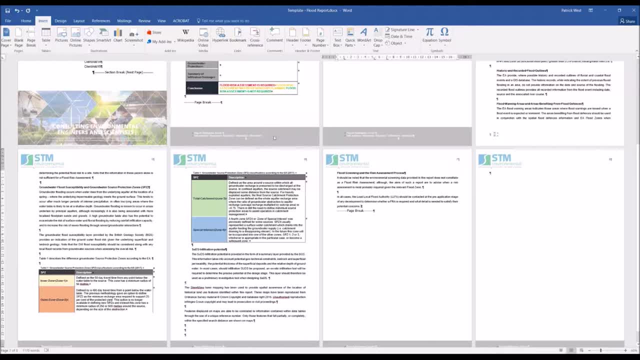 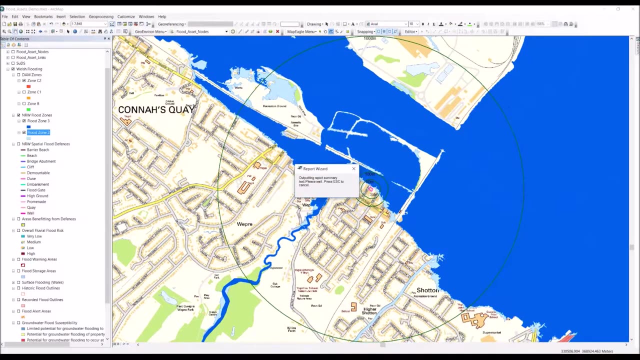 you know, you can obviously put your logos and any internal um sort of nomenclature and systems that you want in there. so that's what that template looks like. um. so we say, okay, i want to use that template, hit okay and the the writer will now go through the layers that we asked for and then we'll. 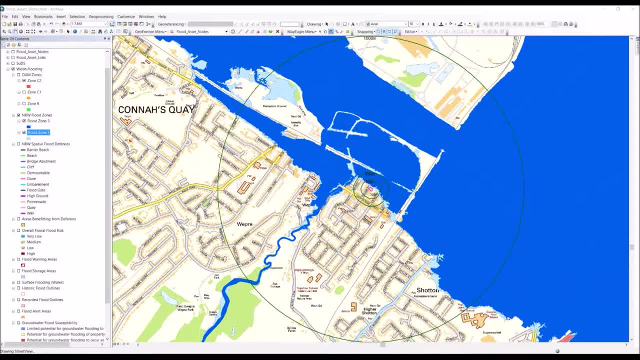 go through the layers that we asked it to search and um and report, and basically generate, uh, the report into the, into that template, and it opens a new word document, obviously using the previous template, um, which i've got up here. you should see on your screen now and what it's doing is it's. 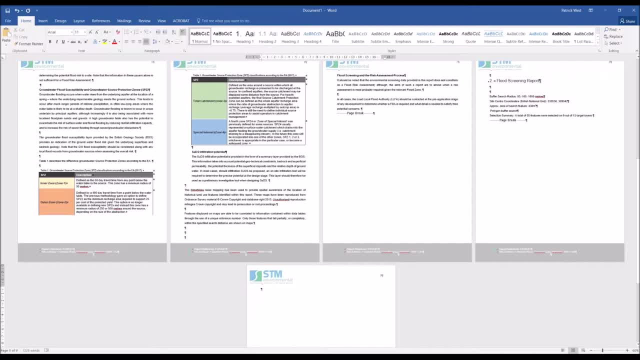 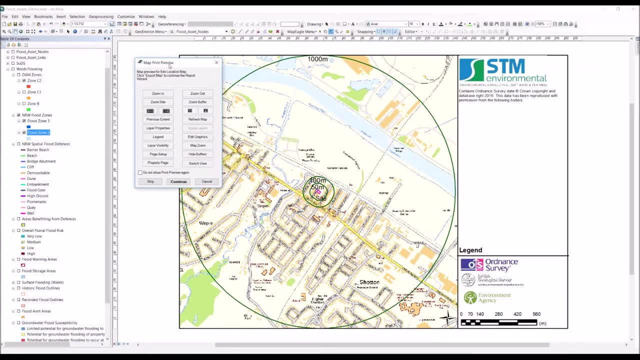 automatically um filling in that report. um, oh, i'm just gonna have to ask to show you um a map preview. so there's an option here. i'm just dragging it from my other screen. i've got to two screens open. you can, you can have a setting. you can see the preview for each map that you want. 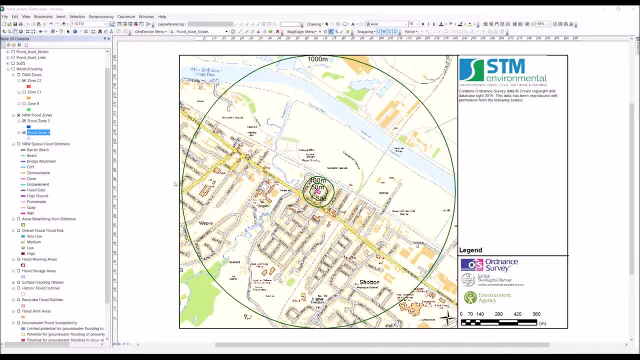 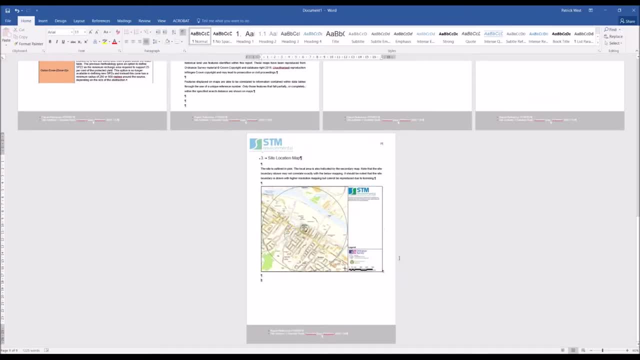 to make sure it looks okay. i'm happy with that. so i won't show it again and let that continue. and i just open back up to my report writer and you can see there it's just populating it automatically now, providing a summary. um, and it's automatically. 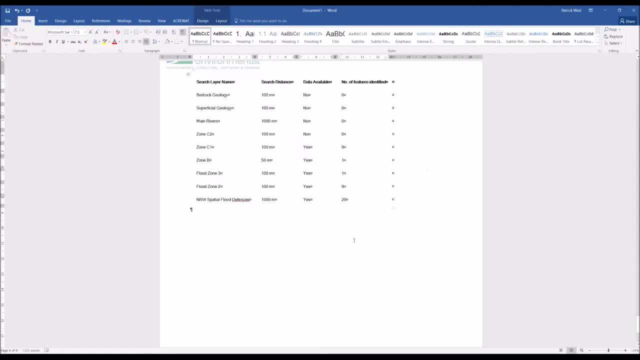 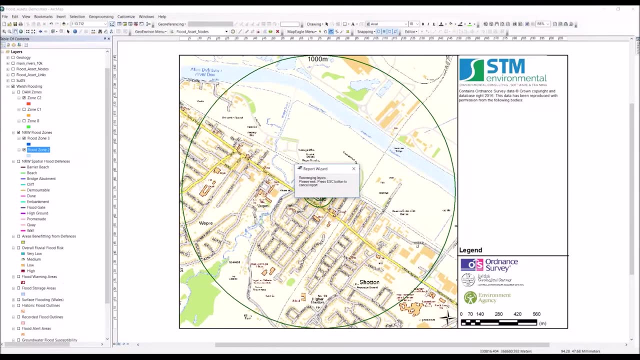 writing that summary, if i zoom in a little bit for you so you can see that, and it's generating that summary we saw there and that might be. as i said, this is the summary report and it's going to finish that and ask me, do i want to continue to a detailed report? so you can see there. so the 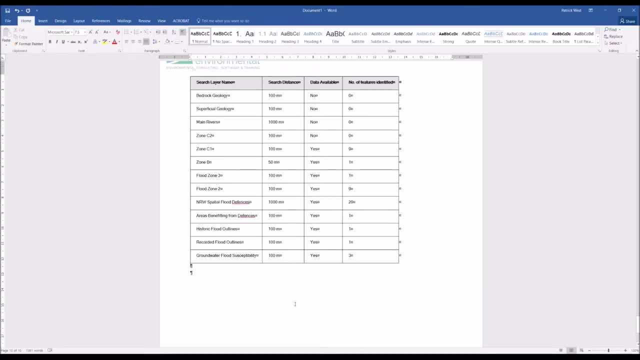 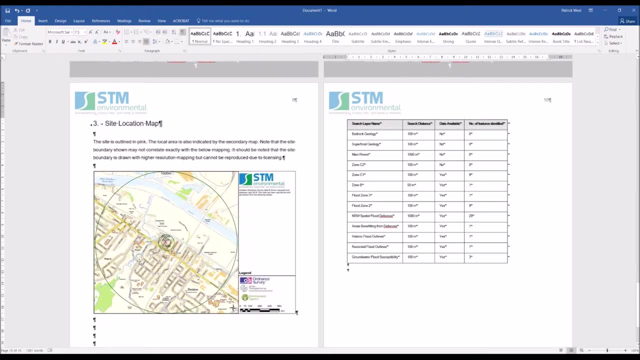 summary report is done, which is on the word document there, and that was. that was pretty quick and it's uh, just generated that report. as i said, you can have all of your. you can have whatever information you want relevant to your authority or your requirements on that map. 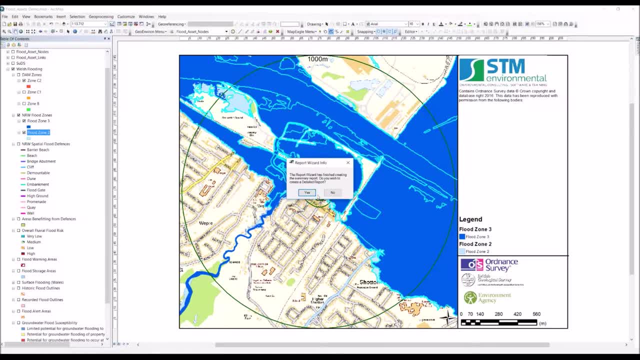 within that summary report. um, and it asks if i want to create a detailed report. so yeah, to make the one the the example that i showed you there. i won't, uh, i won't do that because that runs. uh, i've got quite a few layers and that's going to take sort of 10 minutes. 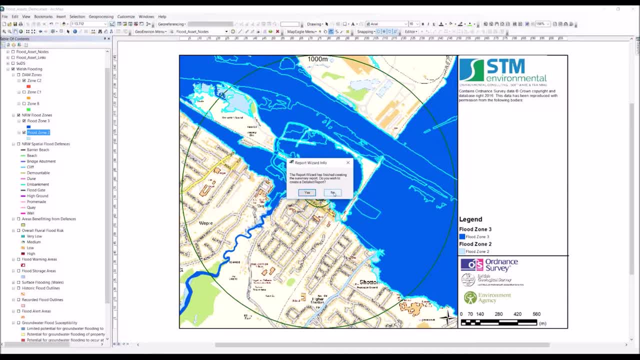 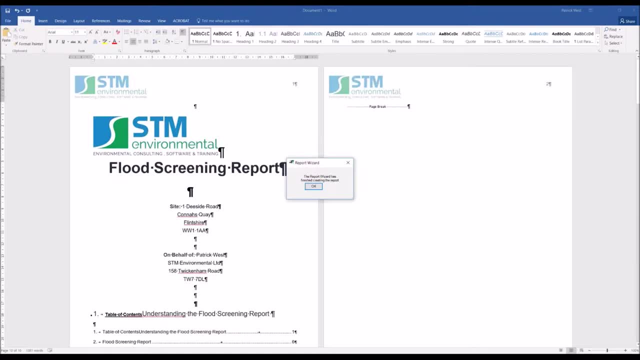 we haven't got too much time left on the webinar, so i'll, um, i'll just i'll say no, i don't want to run a report for that one. uh, and so that's our. and then it finishes the report. there's a, you know it's, it's got a disclaimer. um, oh, bear with me. and the report's finished. so, um, that's obviously our. 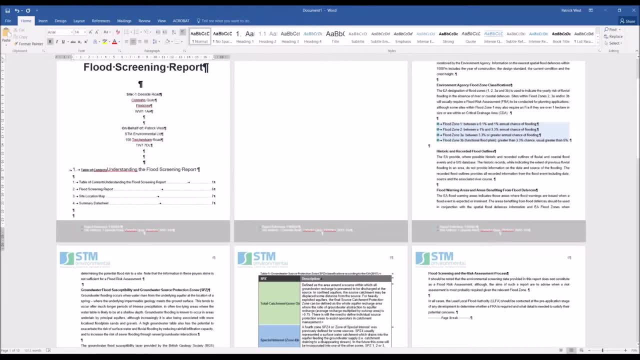 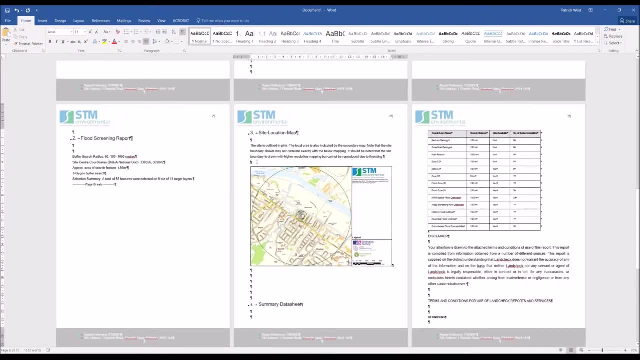 summary report. i haven't put a page break there, so there's a bit of an error, because i clicked in the that was our summary report for that particular site, so you might have your internal screen, as just you know. just to reiterate, if i had pressed uh, continue to the detail report. it. 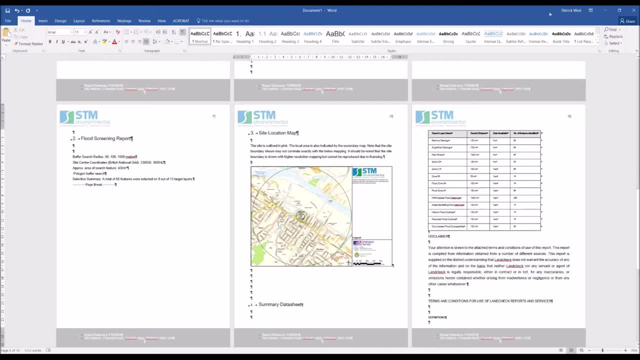 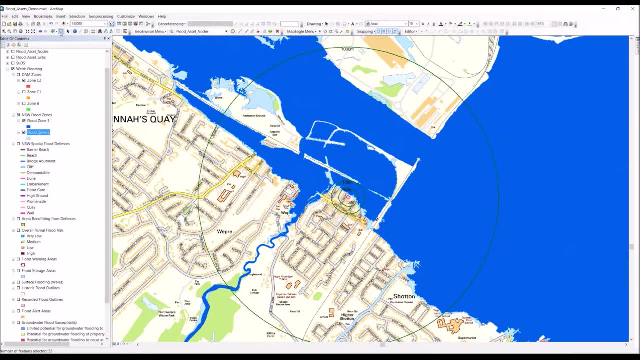 would have given the- uh, the example that i showed so that the um going through all the layers that you want. so we haven't got too much time left on the webinar, so just show you what it looks like to customize those layers. so if we, if you look back on our gis here, um, we can go into the. 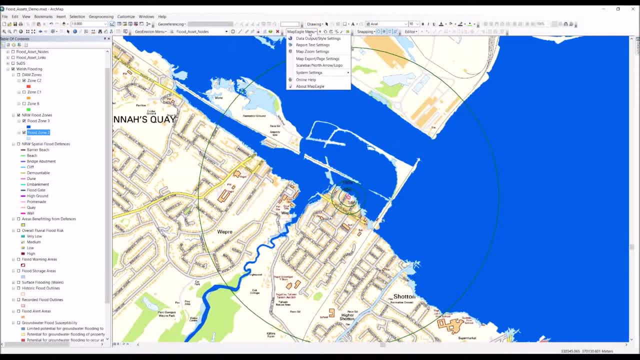 menu, the map eagle menu, and there's a range of options in this and and if you are a current user, you're always free to give us a call and we'll help you out with if you if you don't know how to customize certain features of of your 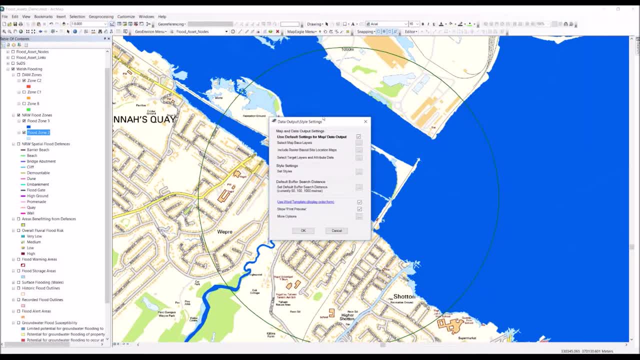 of your um output report and um, this is what it looks like to customize those layers. so obviously you have to have them loaded in your, in your gis map and uh, you can obviously set your base maps and all these. you know various different style settings, but some of the key. 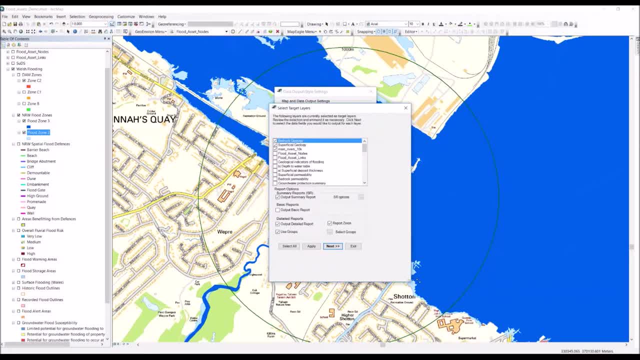 ones, and i think um, we'll start here- is is you choose what layers you want it to look at. so this of the layers that we have in in the GIS, and you, you simply tick those layers that you want it to go through for the search report. so I've got a rivers layer, any geology, and we scroll down. I've 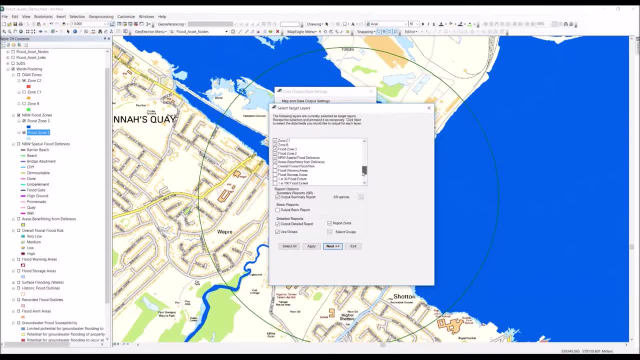 got some flood zone layers that I want to look at and my defenses and any, any records of flooding and and potentially historic records, if they haven't actually gotten the attributes associated with them, and then you can. you can put those layers into groups and if you want them to display, 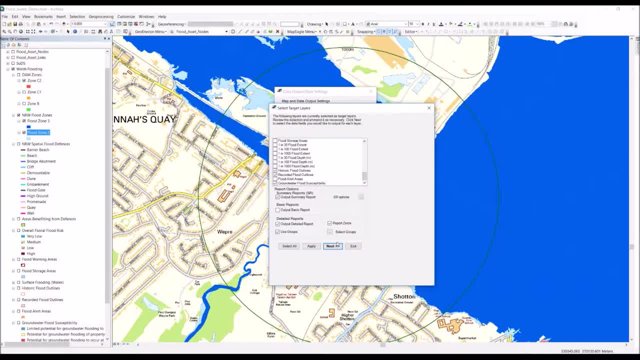 on a map. so you might have a, you know, flood records information, but you might have your own council records, such as sewer records or surface water point records, and you want to display them all in one map. so you can do that if we select this select group function here, which is just. 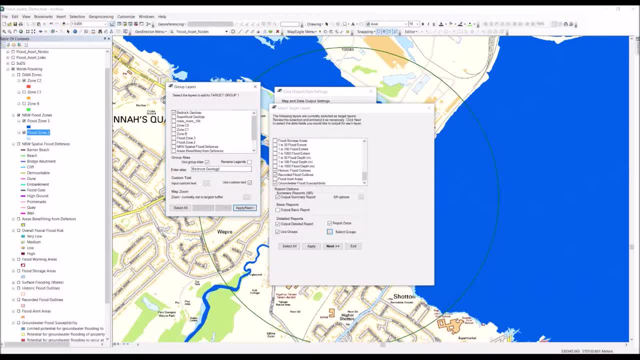 there and it pops up on the other window, and then you can. you can name your group and you can. you can give it an alias name if you want, and you can import custom text, and those text files are saved in a particular folder, and then you can. you can name your group and you can. you can give it an. 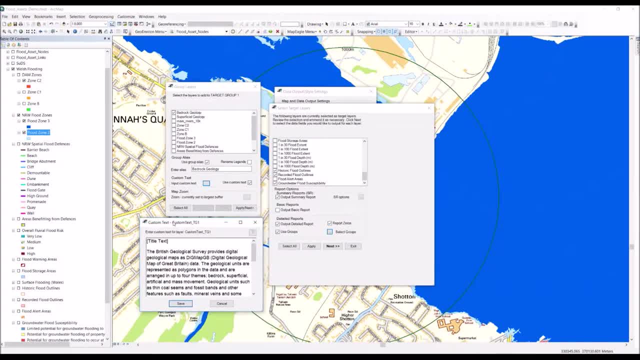 alias name, if you want. so I click that and drag that across here onto the map, onto the window, and there's some custom text for some geology that you can see there. so fully, fully customizable for your, how you want your layers to look, and then you can, you can search through those. so 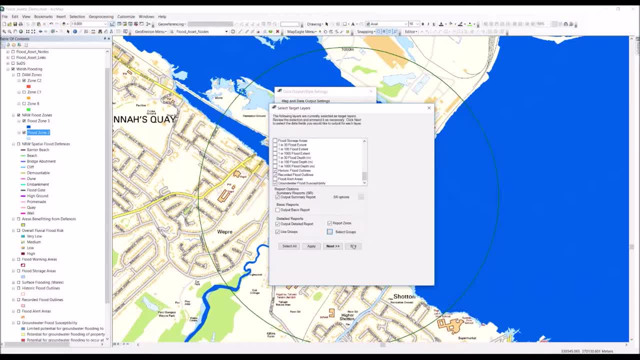 the other. the other key thing, obviously, that's that's in terms of what, what you want to see on the map, but it's probably more important for your internal work, is you want to look at what the attributes are for those particular layers that you're searching. so if we, if we follow next on. 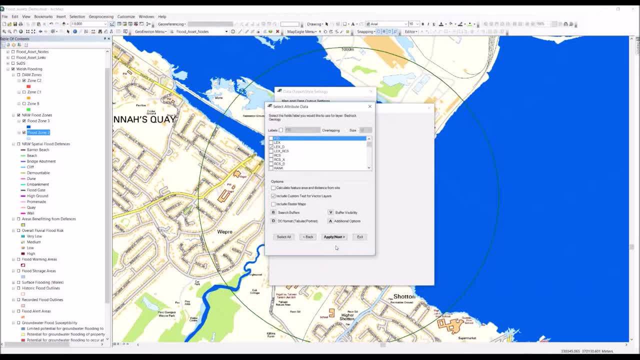 this one and you can. then you get a list of the attributes that are associated with your layer. so, for example, if we, if we just apply next and go all the way to the recorded flood outlines, I think that's a bit more relevant in terms of what the attributes are. well, let's stick to the flood. 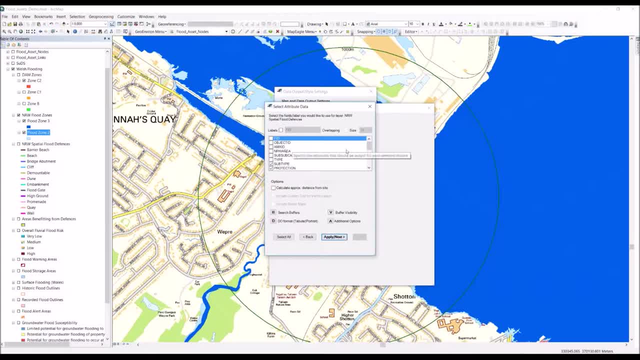 defenses. here's the attribute list of the of the flood defenses, that that that come with that, that shapefile layer, and there's a number of them and I'm going to show you how to do that in just a moment and you can tick which ones you want the report to output. so if I show you the example, if I 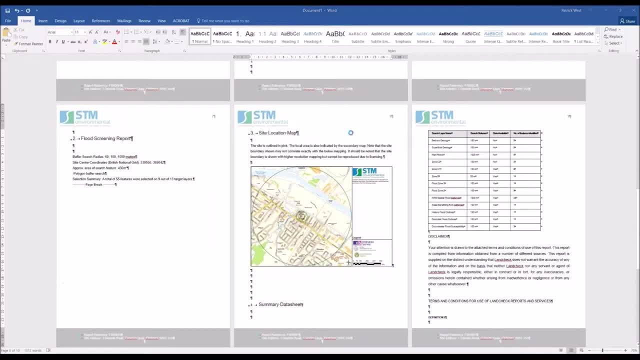 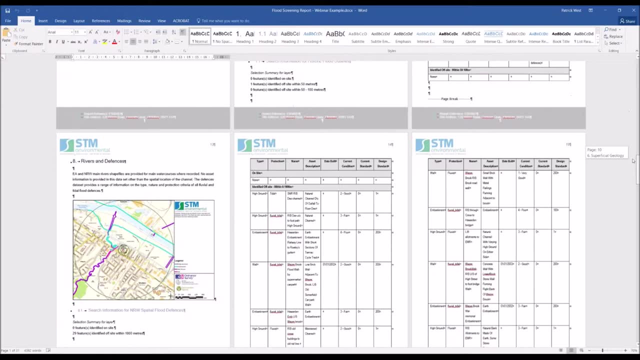 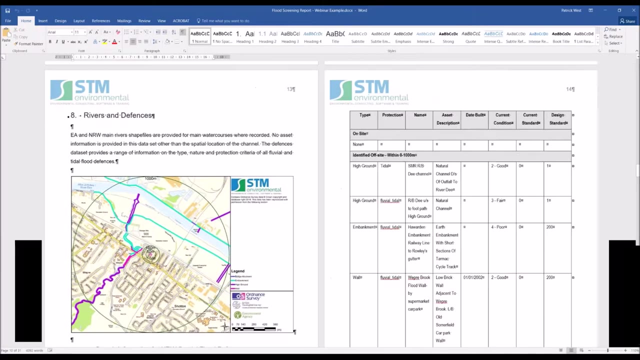 go back to the flood screen report that I made the example, so just pop this up here. so this was, this was the final report, and if we, if we go down to the flood defense section, as I mentioned recently, shortly ago, there's our attribute table and now this table, if you look at the headers on there, 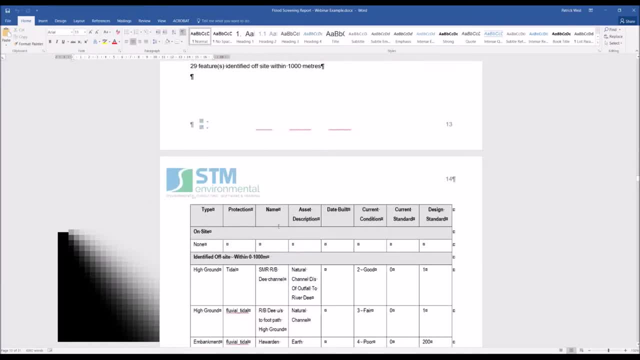 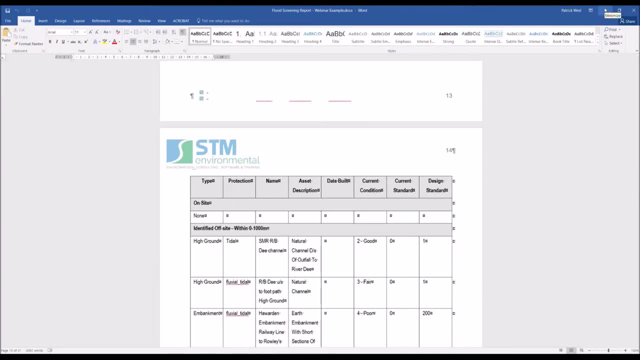 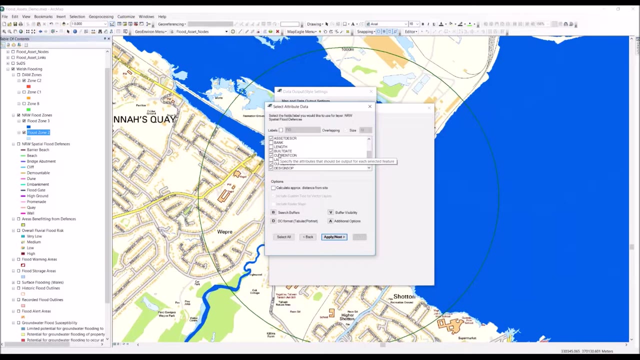 we've had type of the asset, the protection, the description, the name, et cetera, et cetera, any conditions of that defense that that table was customized using. if we go back to the report writer, I customize that using this list, the set of the attributes there, and you can choose what. 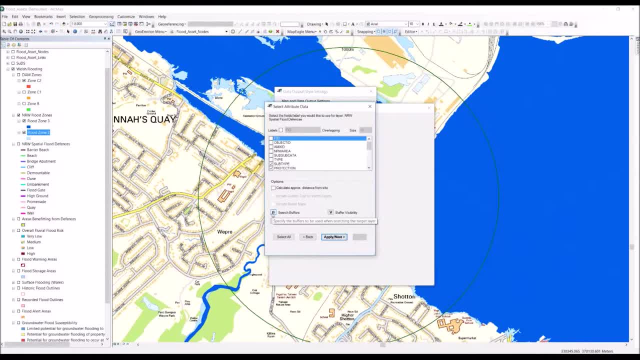 it outputs and obviously you can then choose where, how far it searches, so you can set the buffer distance. so do you want to search within 20 meters, etc? so I'm stressing that point here because I want to make sure you know that it's it's customizable depending on what assets or layers you're trying. 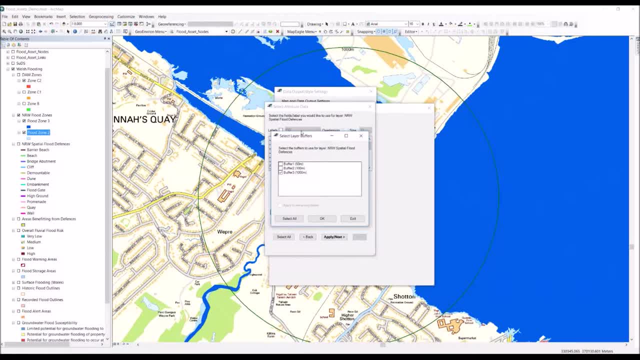 so I've got the, as I said, I've got the flood defenses, searching with 100 meters. but if you've got, maybe you want to look at nearby culverts. you could select the 50 meters to say it radius as well, and so you can find out if you had it, if you had a culvert layer or flood assets layer for your. 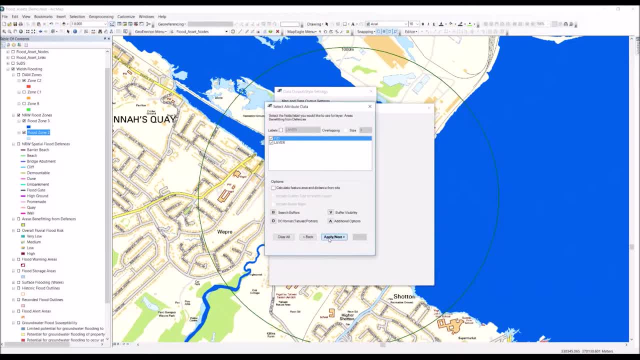 particular authority. so and it takes you through that and you can obviously label. your haven't tick those in these, but you can label your features as well if you want to put the ID. so, for example, I get that this is the recorded flood outlines layer here and I've ticked the name of the flood event, the. 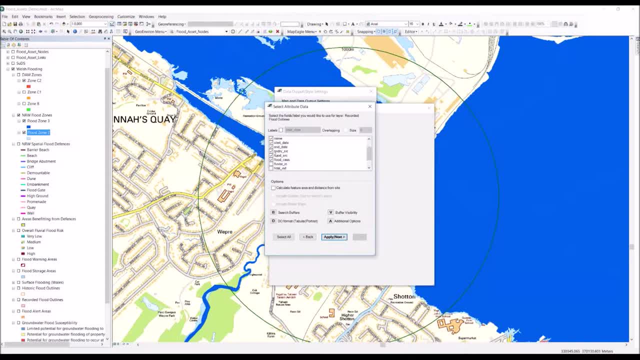 dates- start date, end date, maybe. who defined the boundary? was it the environment agency, was it local authority? and what was the source of the flooding and the cause? so you'll have your own assets, probably an attribute: sorry for them. so you can really, you can really customize that how. 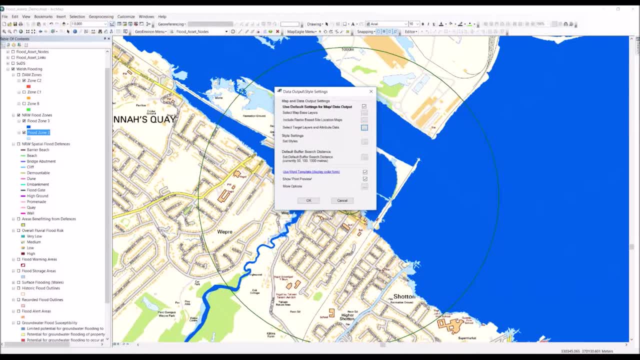 you want it and if you finish that one, so that's how you set up your layers for that and, and as I'm said, there are multiple options for how you want those features to be searched. so you can obviously here set the buffer distance that you want. you might want to search in 20 meters, you can have. 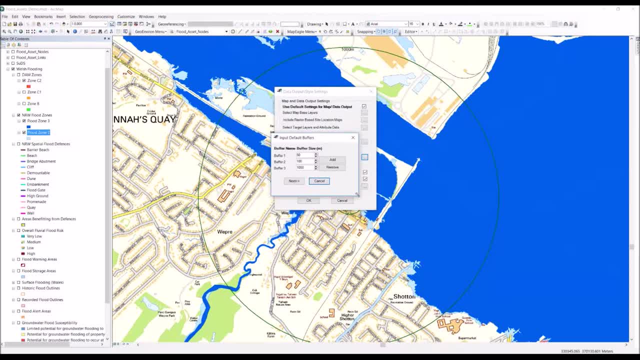 as many buffers as you as you want. there you could just have one. it could just be 50 meters, and you just want to look in the immediate vicinity of a particular point. so that's how you set up the data layers, and I've just got a couple minutes left, so I'll just show you quickly how you would search. 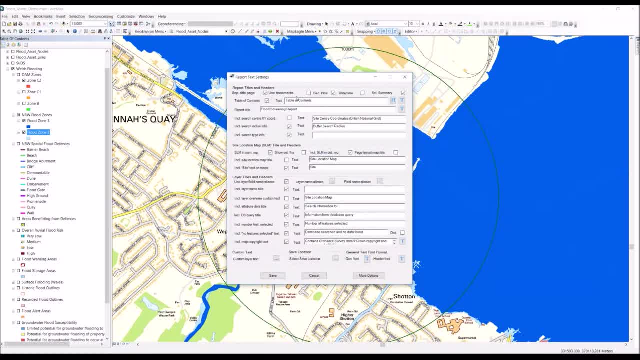 how you would set the report text. so this is: this is how you customize the the report setting in terms of what the text comes out as, and you can actually give alias names. if you see this dialog in the middle here, let's click the mouse, drag it across from the other group. here's the layers that 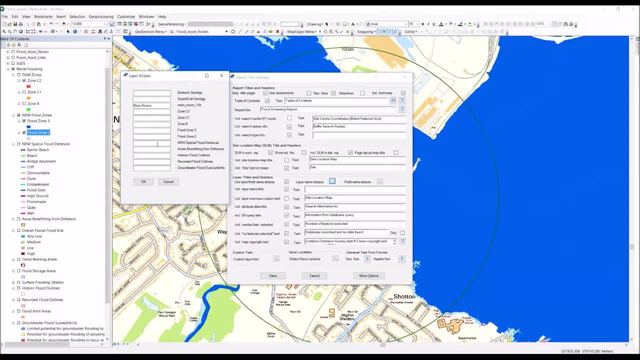 we've. I'm searching for a kind of nice summary there- and you might have a coding for those and you might want to assign them with a, an alias. so this might actually want to be damn, it might be, you know, damn zone, see to it. so that's how you would set the report text. so that's how you would. 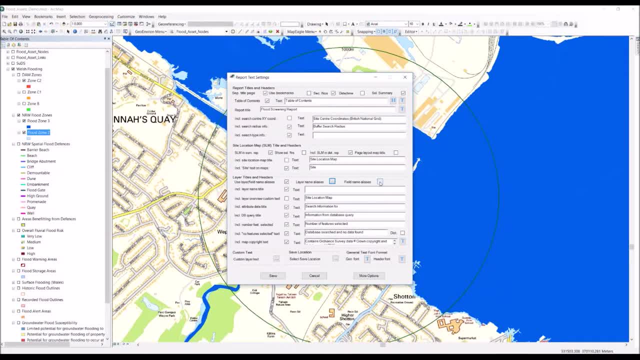 I might want to call it that instead. and you can do that, and you can also give aliases to all those attributes associated with that layer as well. so I know that a lot of the attributes have got quite a kind of unique classification to them. so you can- you can set the aliases for your attributes as 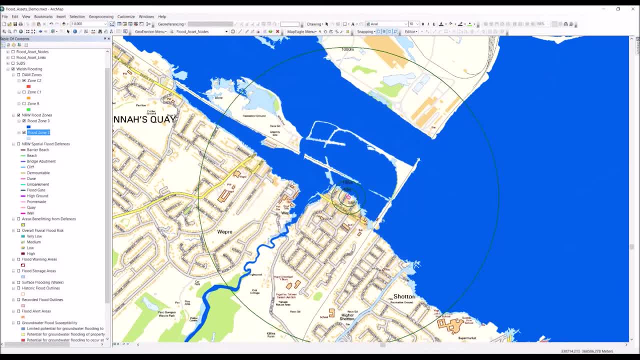 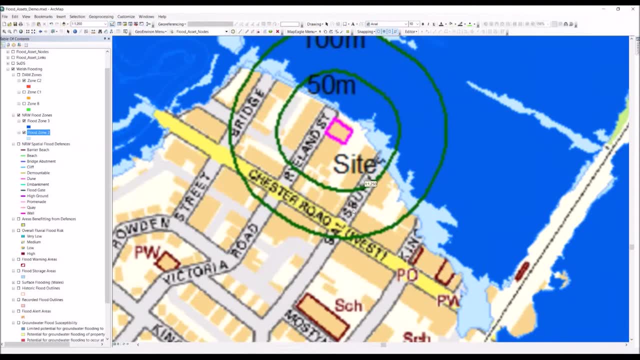 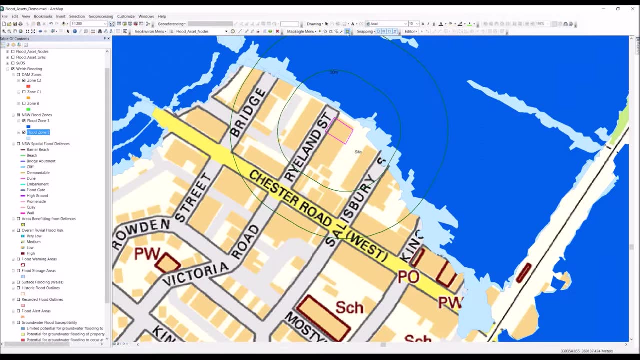 well, okay, so that's a really brief overview of that one. so I think, just just to stress again, I'll show you one more example before we go, of a quick search. so we'll zoom in and both it while we zoom into that site and there and we'll do another search. we can, we can close that previous. 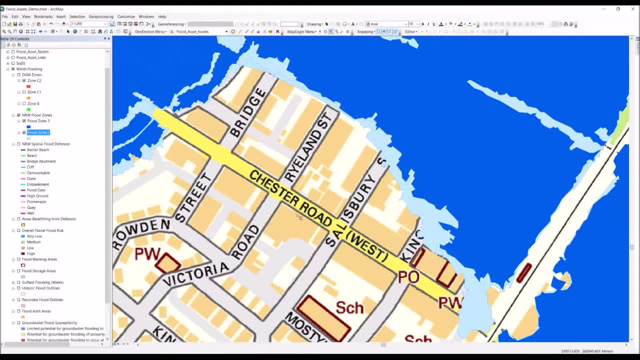 search and we'll do it. we'll perform another one. so say: actually someone's gonna. you want to perform a search? just down the down the road here, which is actually Victoria Road, you can draw your polygon. as I said, you might have a pre predefined site through it, through your database, and, if you can, 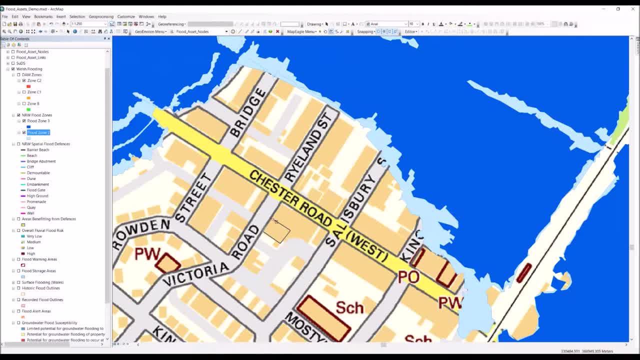 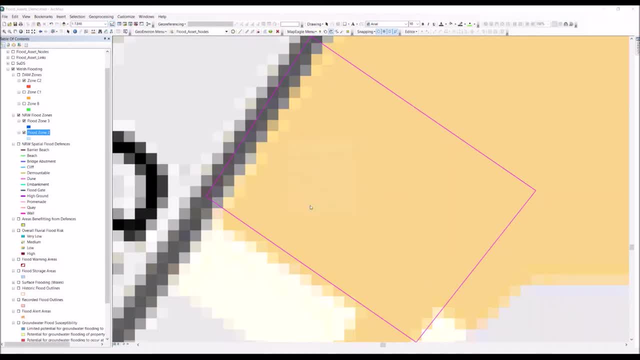 see where them the cursor is there. I'm just going to draw that new site- I'm making that this up- and double click and perform your buffer search so it zooms in, which you'll see there, search the buffer and it will go through those layers that we just showed you on the, on the. 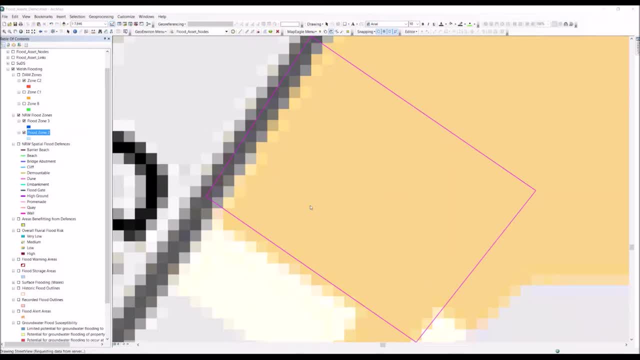 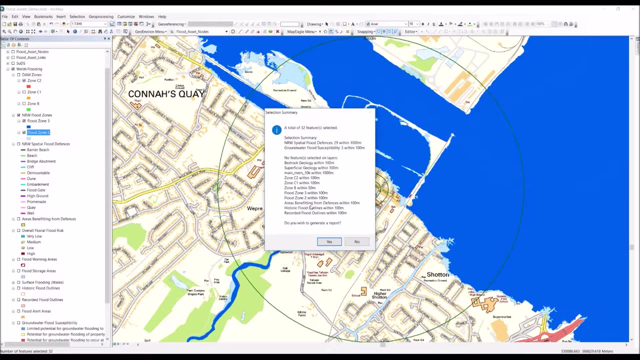 database system where you tried the, the data output system. where you can, you can pick them, so you'll see it shortly. it's about to run through there with it and there you go. it's just a bit of a delay between- yeah, there we are, it's search for all those layers and it's giving 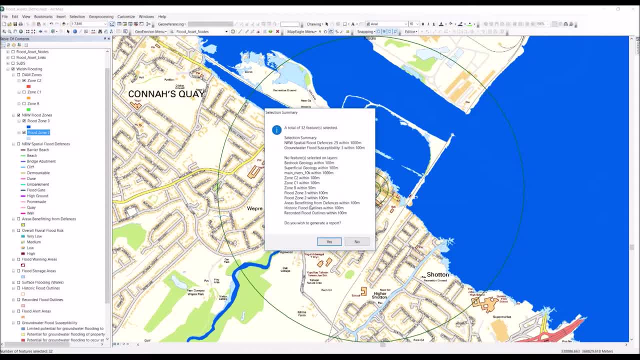 changes there. so it's, it's really really quick for having your, your, your, your initial search and again, you know we can make a summary report from that. so just putting, putting that information you can see there into a table, that might be all you want and a map of your summary, map of all. 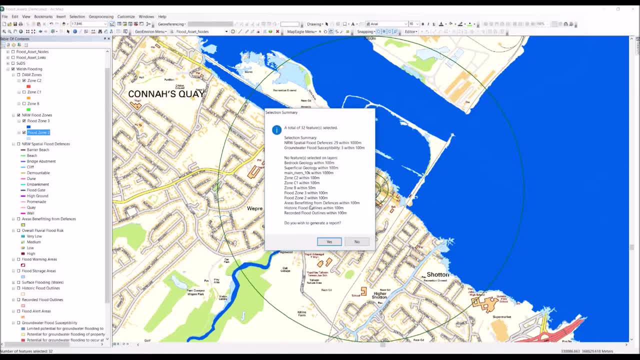 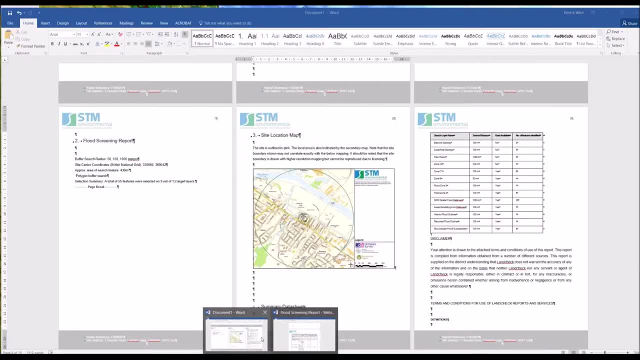 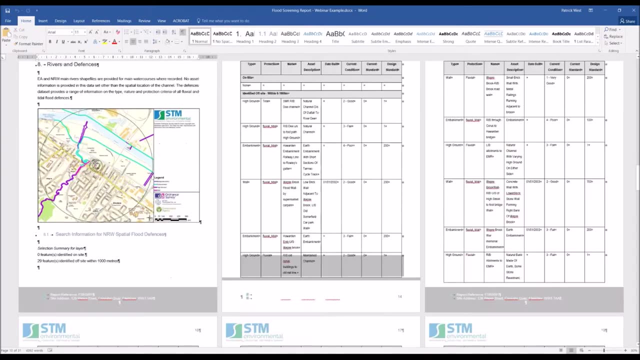 your assets and and geo-environmental layers, or you can, you can go ahead and you can, you can generate your full report. so I'll say no to that one and and go back to the. go back to the final report. that sorry, the final report here, the flood screening and, uh, and hopefully, 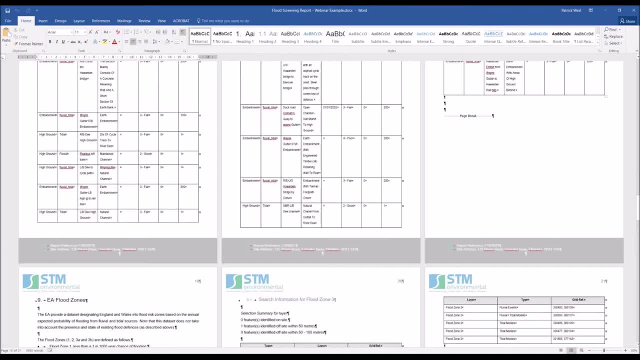 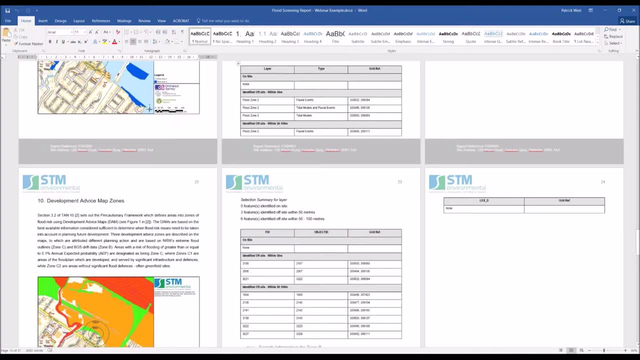 you, you can get your reports to look like this. as I said, if you are a current user and and future users, there's there's plenty of help here to um to try and get that, to customize how you want it to look and how you want and make sure you get the right the information out of it. so 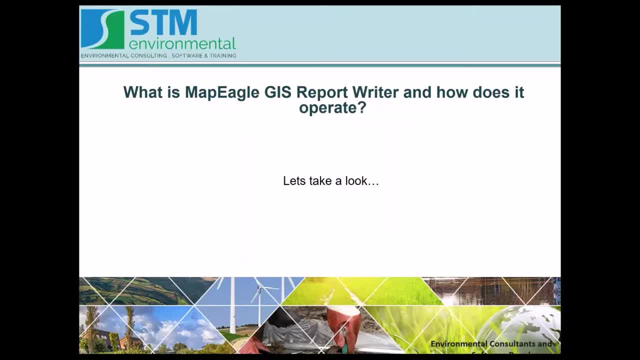 um, if we go back to the PowerPoint, just to sort of wrap up, um, I know that was a bit bit brief, we only had 30 minutes there. so, um, please contact us if you, if you want any more information- and this is being recorded so you can- you can request a copy of this. 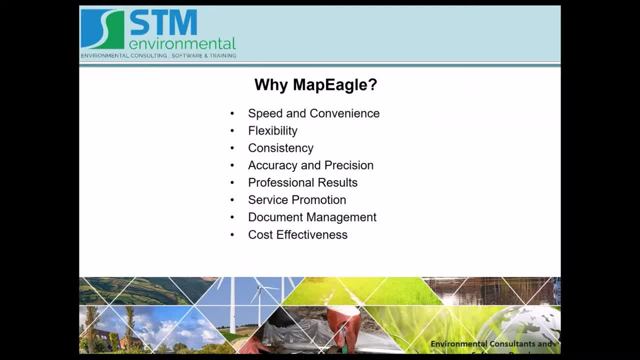 video. um, yeah, if you want to show any colleagues um or you for future reference. um, so so the, the, the report writing tool and the screening tool is is meant to make your um searching process a lot more um, efficient and potentially more effective. so it's obviously quick. um, hopefully I've showed. 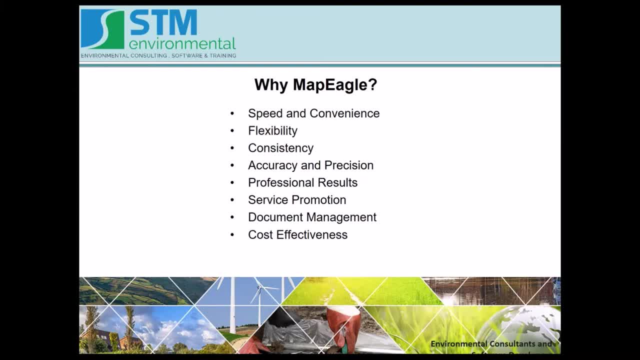 you. it can search through your the layers that you want um very, very quickly, and those are all customizable, which is the important part. so, depending on what information you have and what's important for your search request, you can choose that and you can choose all of your buffer. 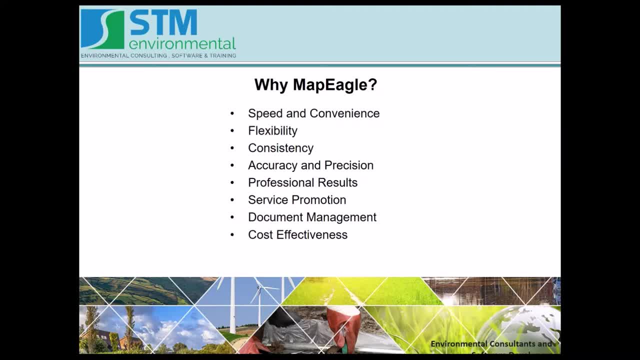 distances and your um, basically everything that you want to uh to do. you can customize that um, but it's also has a potential to be used for internal and external documents and and reporting um. internal um summary reporting- uh yeah, quick screen, or you can use it for potentially pre-app. 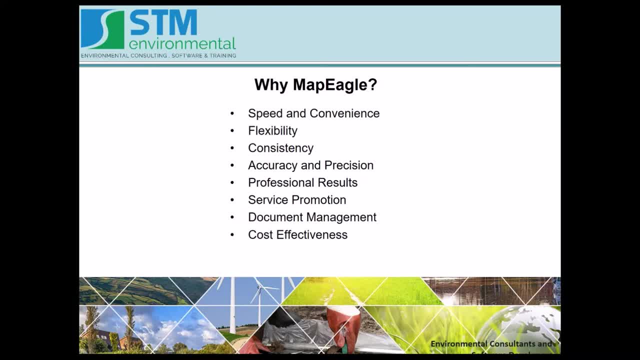 work. so, you know, providing people with an environmental search um to give them a bit more information, and hopefully I know that some authorities um do charge for that sort of information um, and that's, uh, obviously a very effective way of getting that report done quickly. so it's obviously more effective than searching through those layers, um, and it's potentially more.